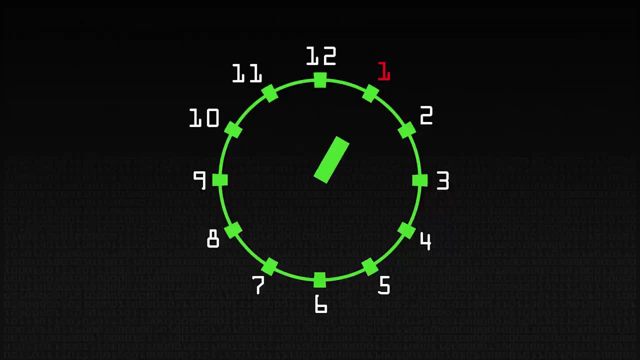 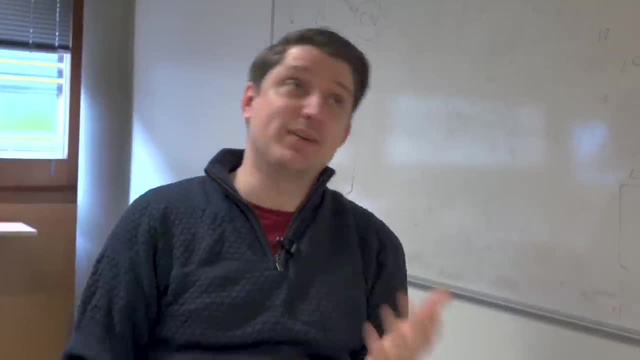 Yeah, you go all the way around to 12 when you start back at 1,, 2,, 3.. It's that, but obviously your numbers are bigger. There's many more hours in a day. Even if you calculate this modulus, this is still a difficult sum because you have to do 23 times 23 times 23 times 23. 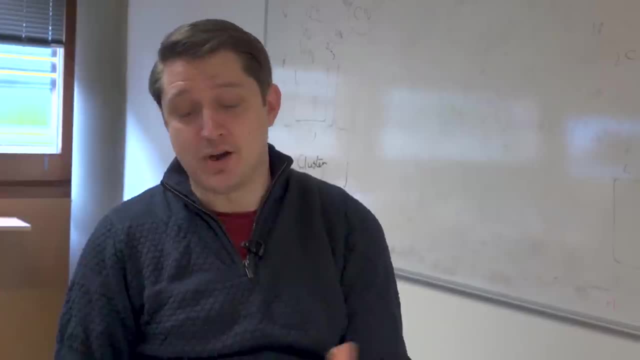 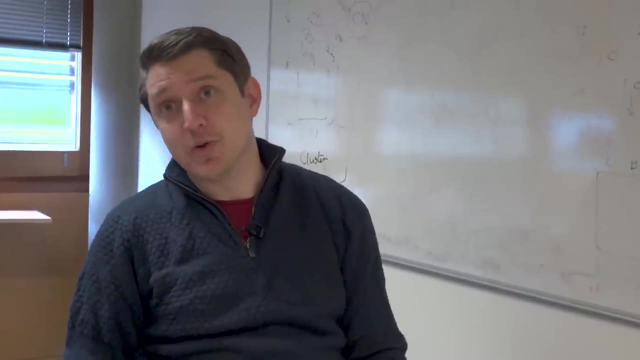 373 times That's. that's not very fast, right? And if 373 was a 600 digit number, then even by taking mod, there's no hope of doing this, right. So we need some kind of algorithm that calculates what we call an exponentiation. 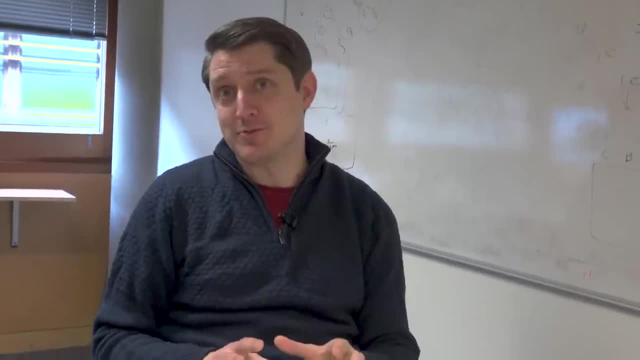 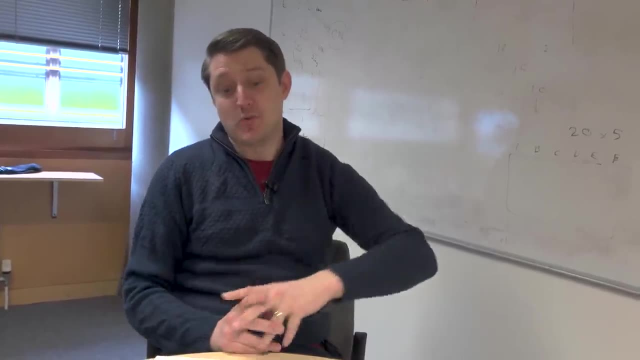 much, much faster. And that is a square and multiply algorithm- Really neat little algorithm, I think, fairly intuitive to understand And it's used all the time in computer science. Whenever you have a sum like this, which is a lot of the time, you can do it really, really quickly using square and multiply. 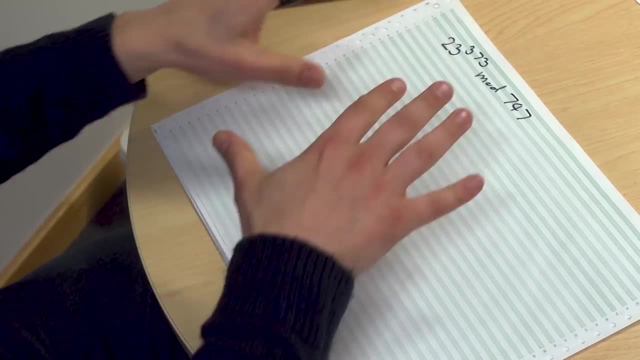 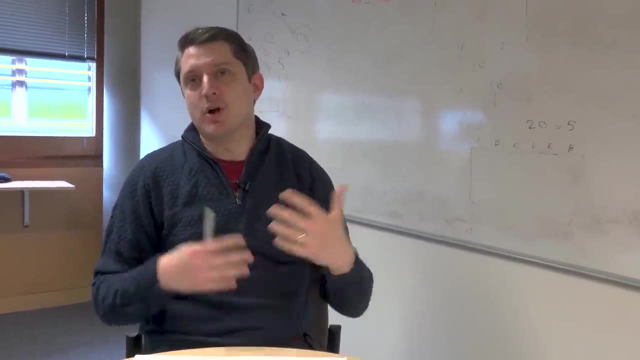 Now, actually, as it happens, they picked quite difficult sum. right, There's reasons for this and we'll go into them, but I'm going to pick a slightly easier sum. Perhaps the first thing to do is to look at how the square and multiply algorithm works- sort of an overview, right? 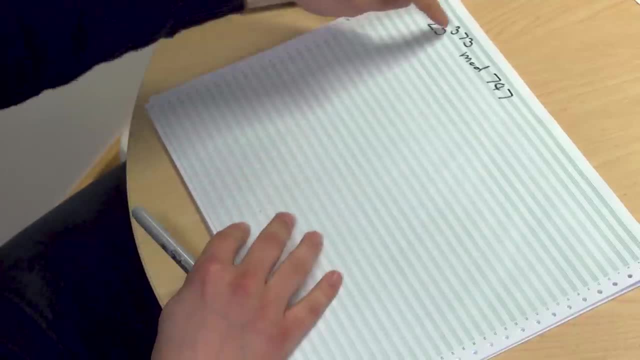 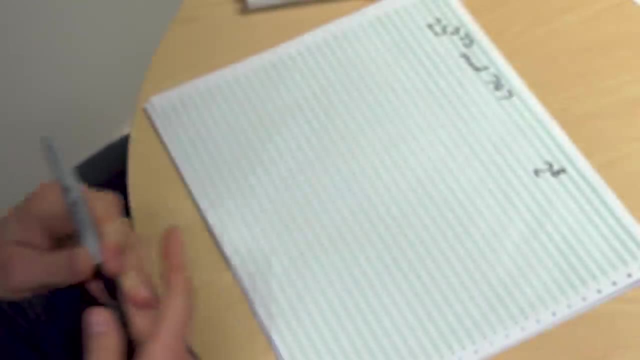 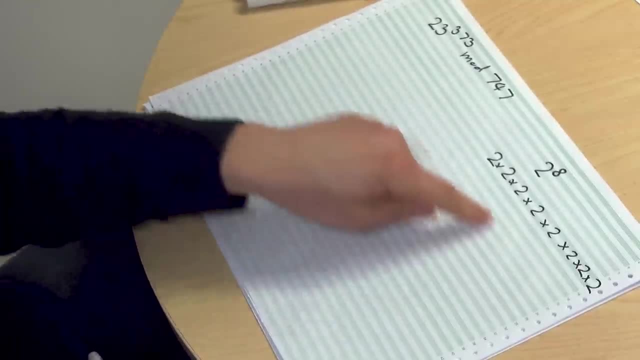 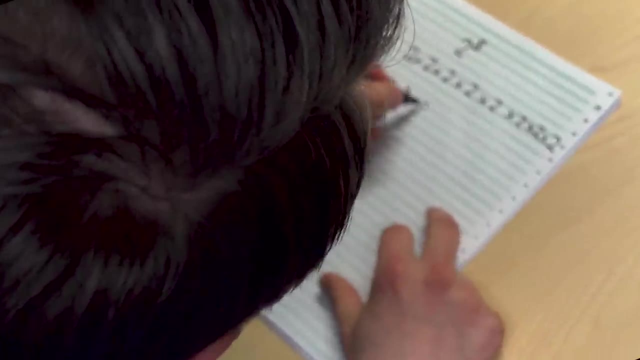 How many is that Times 2, right Now. that took me a fair while to write out, but actually you could save yourself a little bit of time because you could do 2 times 2 is 2 to the 2, right, It's 2 squared. right, Then 2 squared. 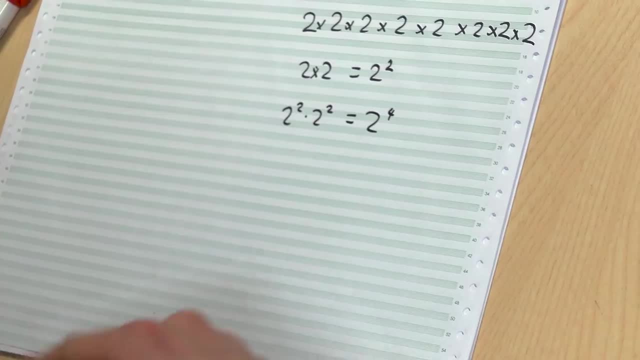 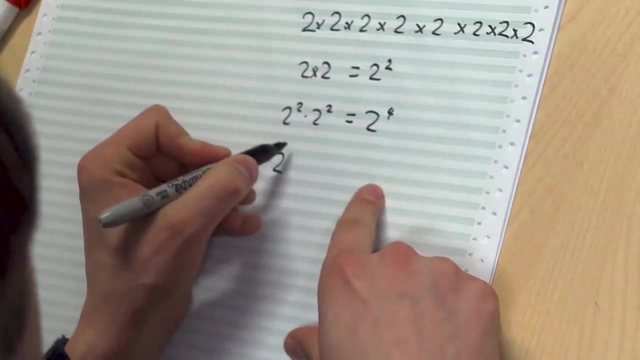 times by 2. squared is 2 to the 4.. It's 2 times 2 times 2 times 2, right. And then, if we do square this again, we can go, we can jump all the way up to 2 to the 4.. 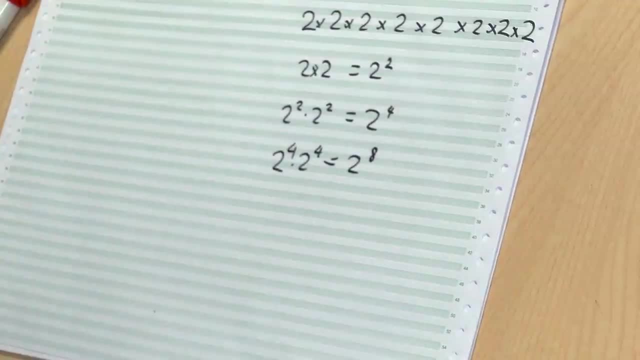 2 to the 4 is 2 to the 8., And so we can actually do it in 1,, 2, 3 operations. We can get to 2 to the 8 instead of this 7 or 8 operations. 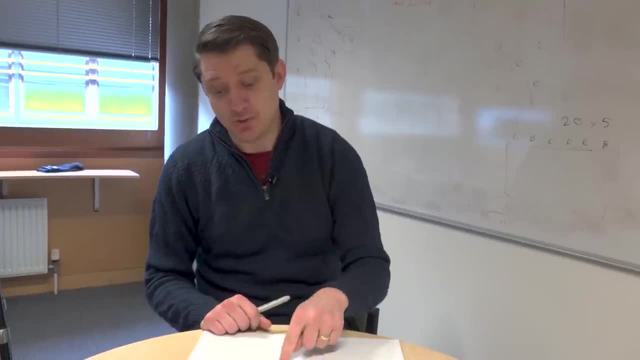 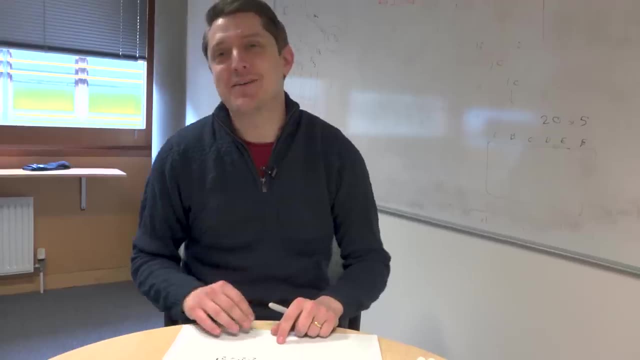 If, instead of multiplying by your original value every time, you multiply by one of these much larger intermediate values, you can much more quickly converge on the solution you want. Assuming it's a power of 2, right, We haven't dealt with the slightly prickly subject of what happens if this isn't just a power of 2, which unfortunately 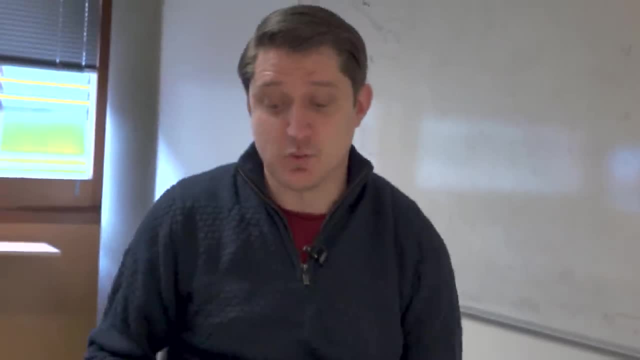 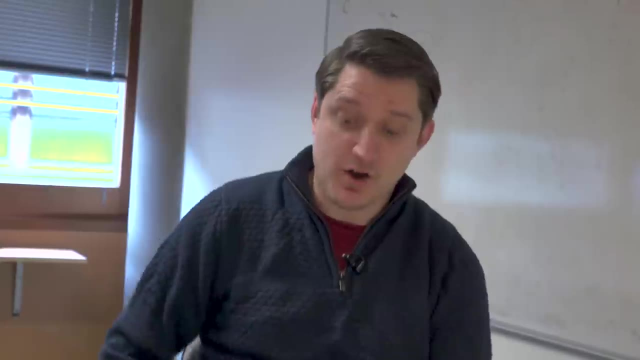 in cryptography is most of the time. So in principle the idea is that we can sort of jump forward in powers of 2 or you know, by squaring much more quickly. But we need some kind of mechanism of what we do if we're not just going to get there by squaring every time. 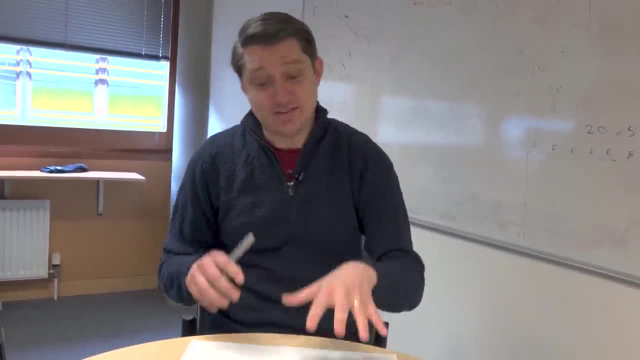 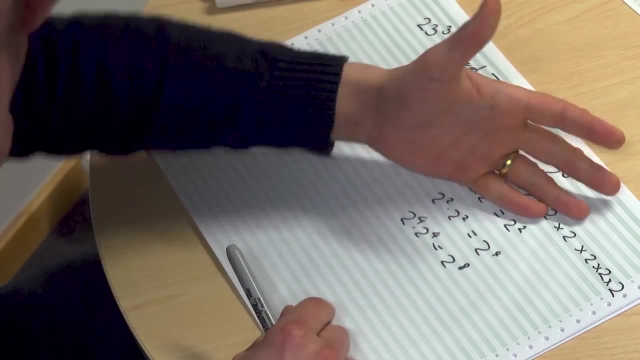 What we actually do is we do something called well, in this case, we're going to look at something called left to right, square and multiply, And the idea is we look at the exponent 373 or 8 or some other number and we represent it in binary and work out what operations we're going to need to do. 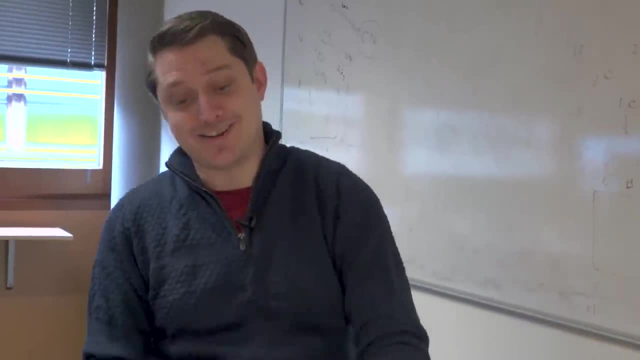 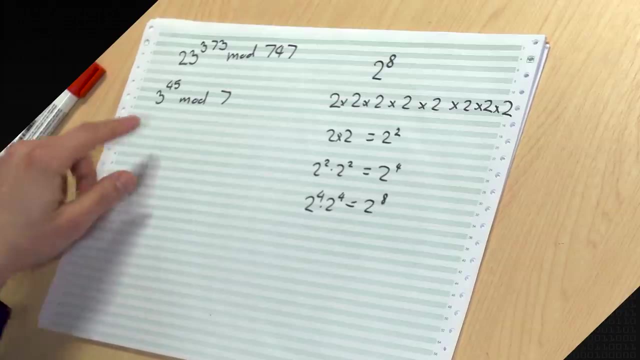 to get to the right result. I'm going to use a slightly smaller example of this. otherwise we're going to have to bust out their pocket calculator. So we're going to do 3 to the power of 45 mod 7.. This is a strange sum because in some ways 3 to the 45 is an extremely large intermediate value. 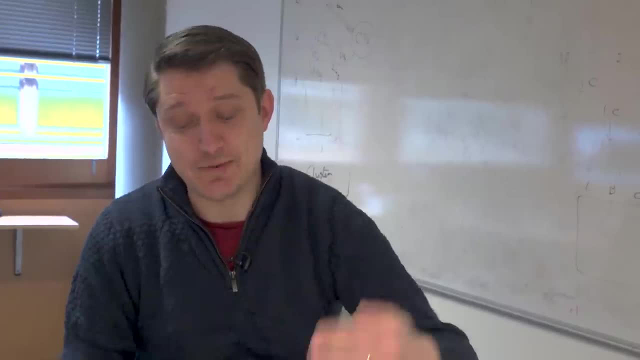 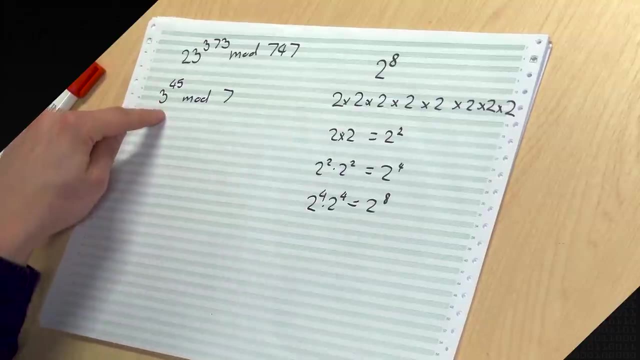 So we want to reduce mod 7 as much as possible so that we keep it small. Otherwise we get a huge value and we end up with just a number between 0 and 6 anyway. What a waste of time that was. But we can also use square and multiply to make this much faster. 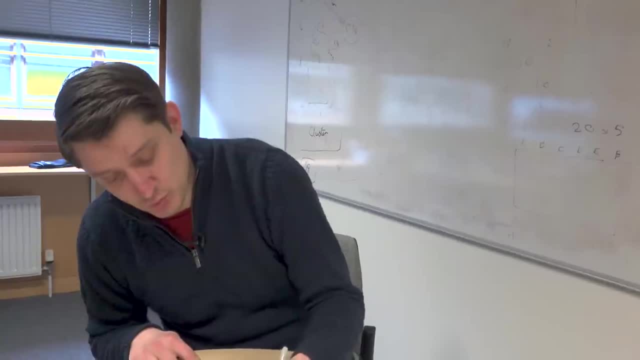 So the first thing we're going to do is work out what 45 is in binary, and that's 1 over 0.. 1, 1, 0, 1.. I'm going to draw a line here so we can have some sort of delineation. 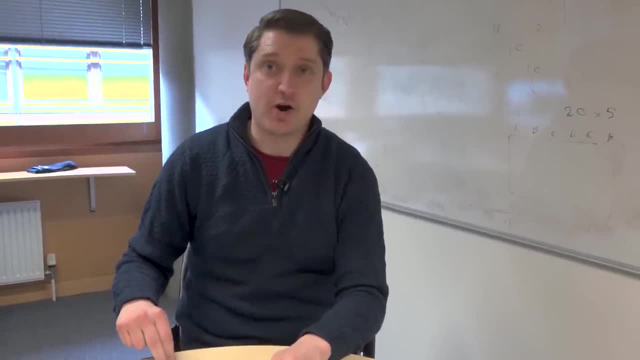 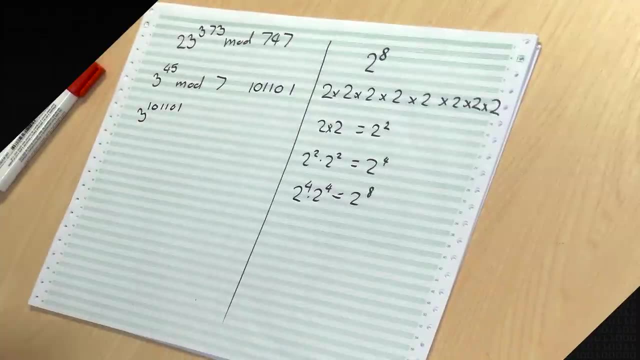 Now a couple of things to think about. is suppose we treat this exponent as binary, So what we actually want to do is calculate 3 to the 1, 0, 1, 1, 0, 1.. Whereas this is a decimal number and this is a binary number. so that's slightly confusing. 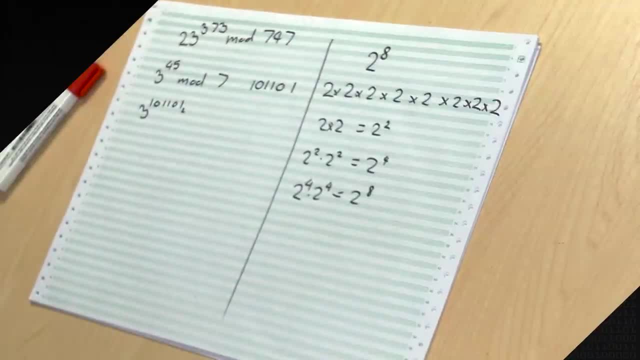 I'm going to write a little 2 in here to show us it's base 2.. But a couple of things to think about. Suppose you have x to the 1 times by x to the 1, that's in binary, Alright. 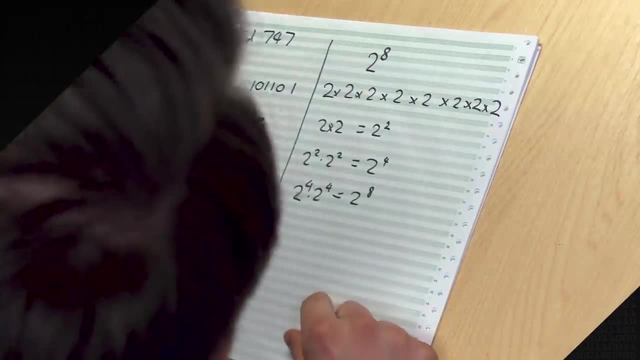 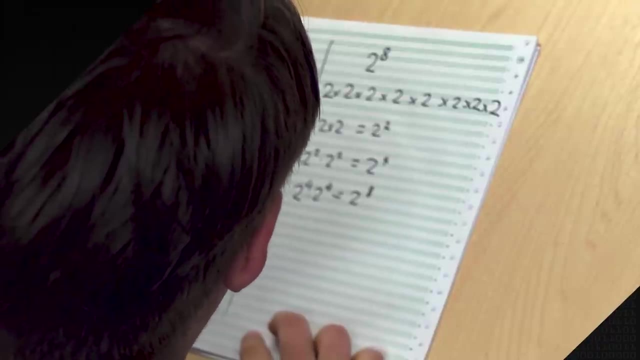 So if you get x squared, you're going to add these two ones together, so you're going to get x to the 1, 0.. If you do x to the 1, 0 times x to the 1, 0, so that's x to the 2 times x to the 2,. 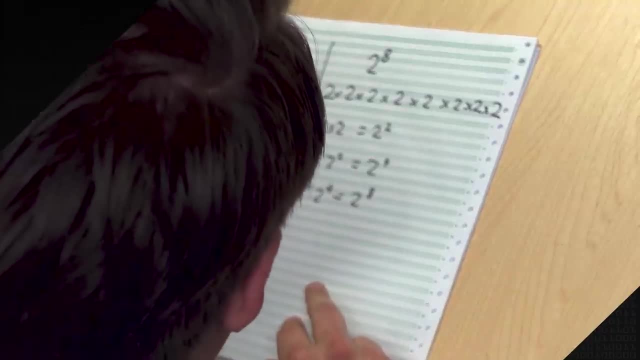 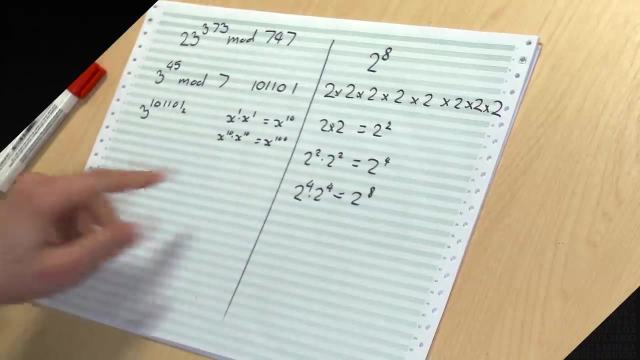 you're going to get x to the 4, it's actually x to the 1, 0, 0.. So whenever you square a number, your exponent shifts left one bit. it doubles in size and shifts left. You just stick an 0 on the end of it. 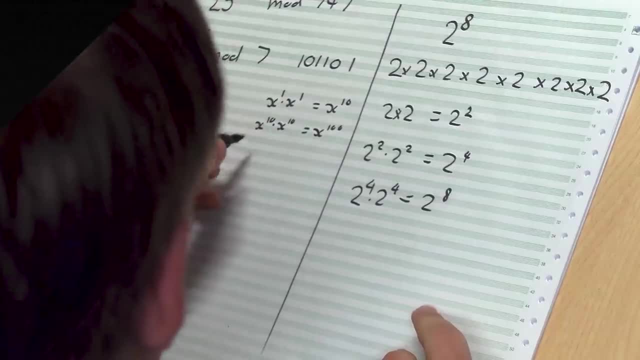 A 0 on the end of it, Right, And you multiply it by the original number. So if you take, for example, x to the 100, right, it's not 100,, it's 1, 0, 0.. 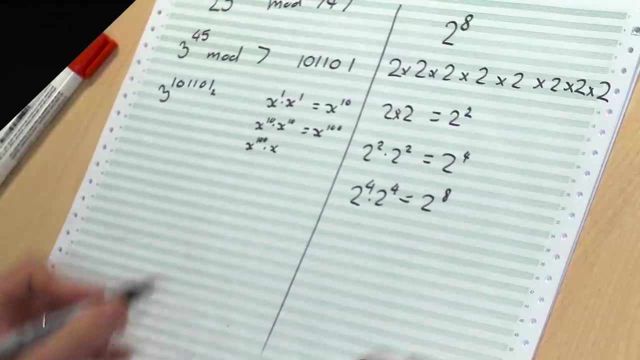 If you take x to the 1, 0, 0 and you multiply it by the original x, that's actually just 101.. So it's x to the 1, 0, 1.. Right, So you've got two rules. 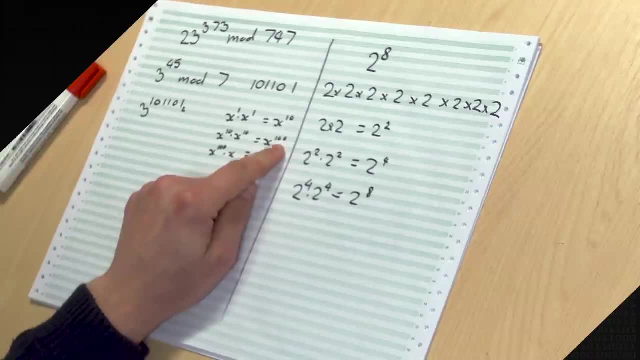 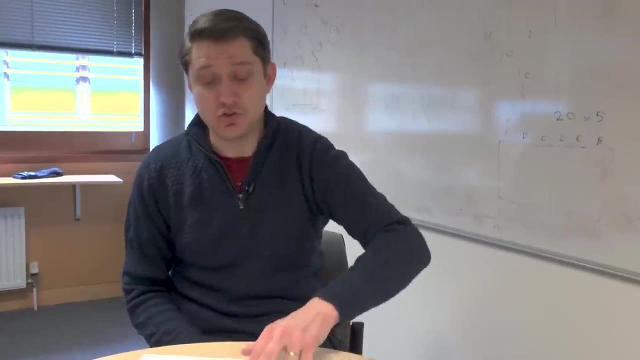 If you square a number, you take its exponent and you add a 0.. If you multiply the original number by your intermediate result, then you just add 1 to the exponent Right, And so, using those two different, square and multiplies. 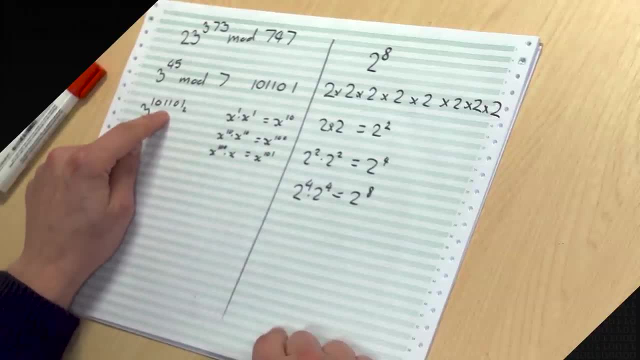 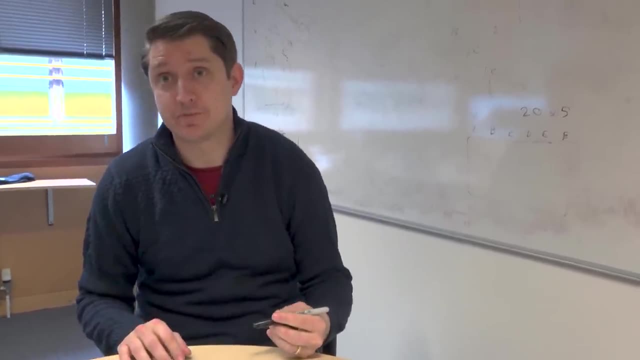 Right, We can recreate this exponent here in the minimum number of steps, So it might be 3 squares and 2 multiplies, Exactly, Yeah, And you have to do them in the right order as well, Right? And so what we're going to do is we're going to build up this exponent here or this one. 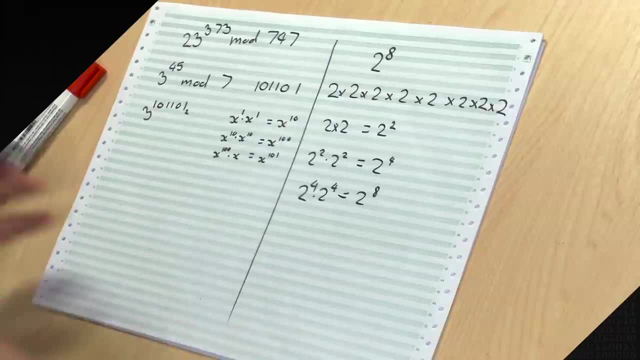 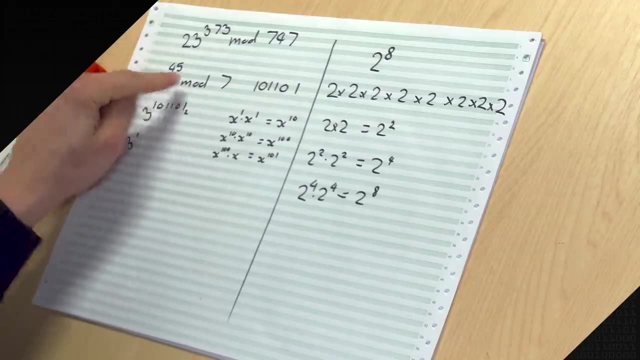 here by doing repeated square and multiplies in the correct order, Right. So let's start with 3 to the 1, right, which is 3.. And what we want to do is now do 3 to the 45, mod 7.. 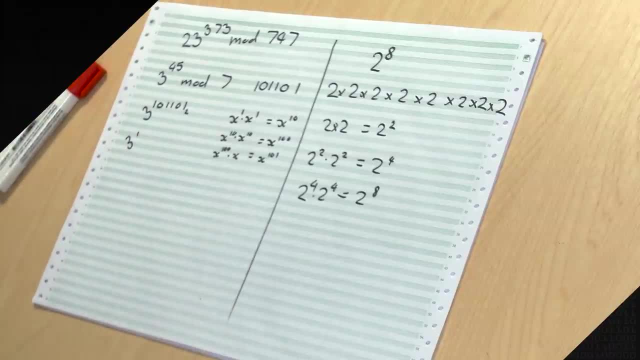 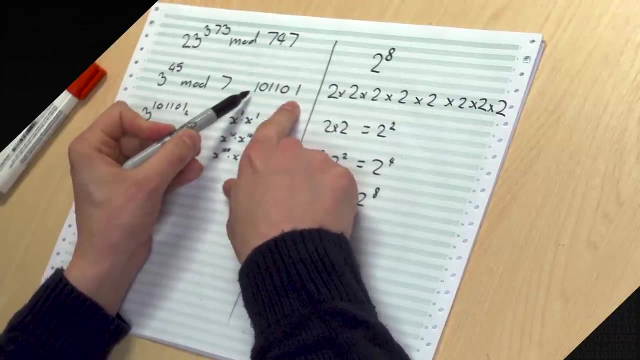 Now, I'm not going to calculate the actual values for a minute. We can fill them in in a moment, Right. But the first thing we want to do is we want to go from 1 to 1- 0. Right, We're going from left to right in this particular version of the algorithm. 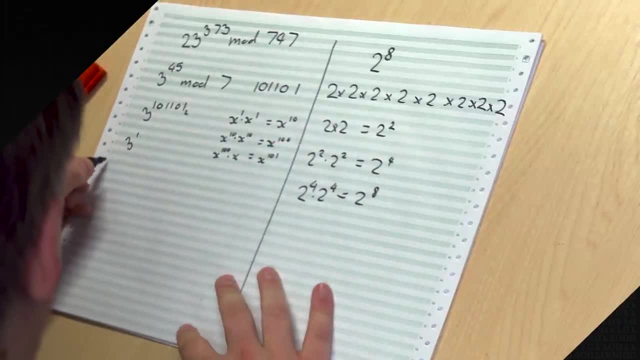 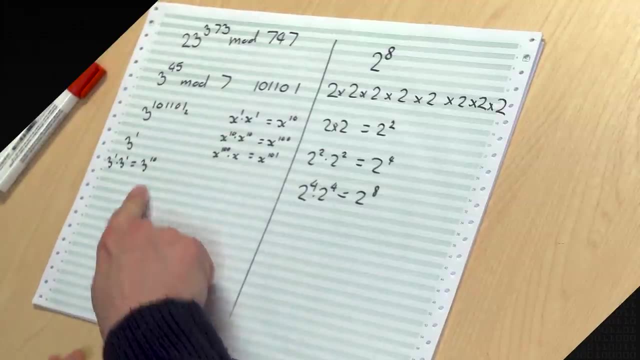 So to do that we need to square it. So we do 3 to the 1. times by 3 to the 1 is 3 to the 1- 0. Right, So that's actually 3 squared, Right. I'll tell you what. 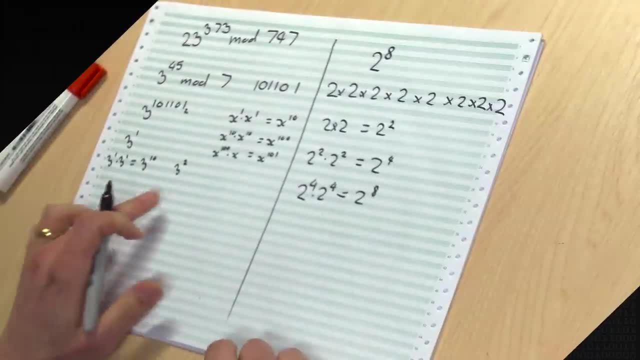 I'll write in 3 squared here, so we can keep a track of what the number is in decimal. So this is our binary, This is our decimal. Now we want to go from 1: 0 to 1: 0 1.. 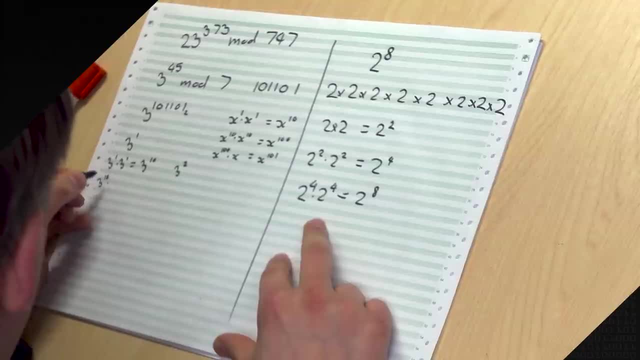 We can't do that in one step, Right, So we do square first. So we do 3 to the 1: 0, 3 to the 1. 0 is 3 to the 100.. Right, That's 3 to the 4.. 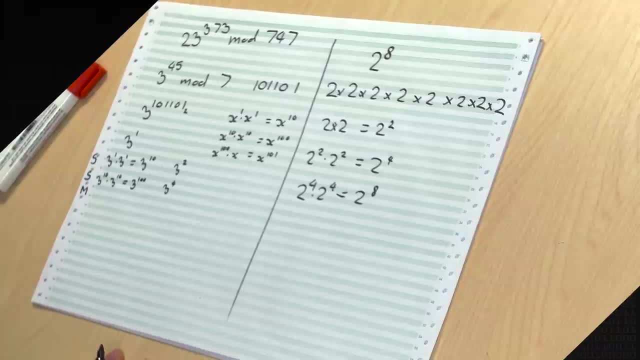 So this is a square, This is a square, And now we're going to multiply, And I've sort of not left myself a huge amount of room here, but we won't worry about it. So 3 to the 1, 0, 0 multiplied by 3.. 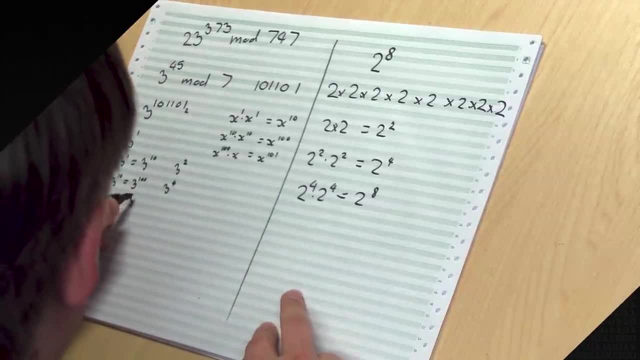 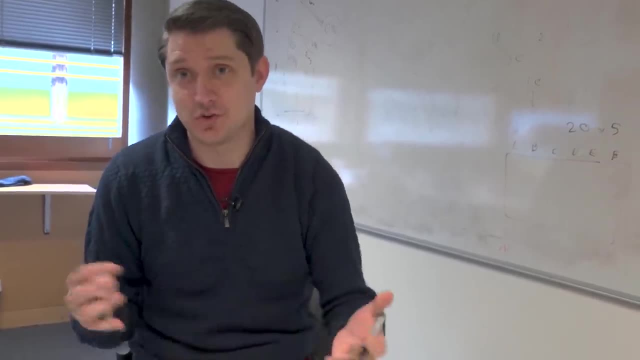 So the original value that we have at the top is 3 to the 1, 0, 1. That's 3 to the 5.. Right Now we're nowhere near 3 to the 45 yet, but hopefully you can see we're sort of making. 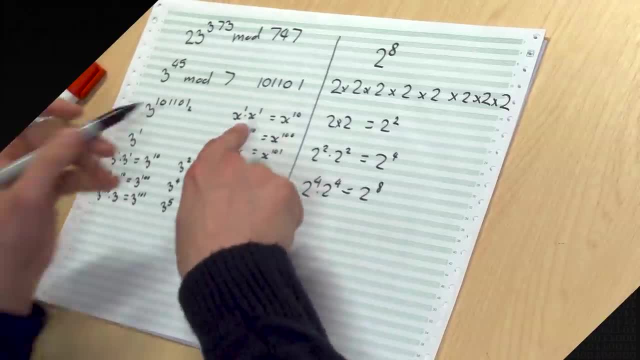 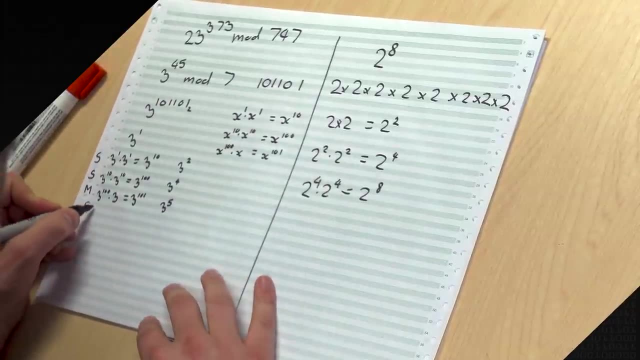 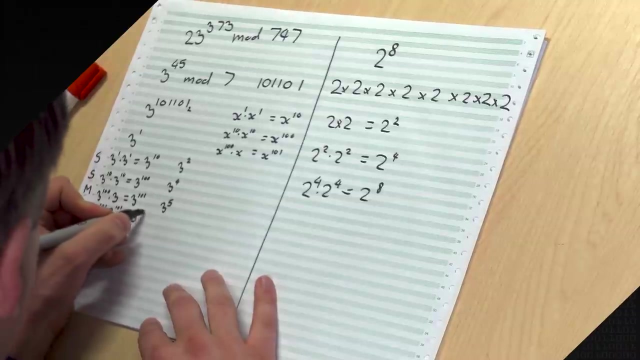 some progress, Let's keep going. So the next one: we want to go from 3 to the 1 0, 1 to 1 0, 1, 1.. So we need to square again, So square, So that's going to be 3 to the 1 0, 1, multiplied by 3 to the 1 0, 1 is 3: 1 0, 1, 0.. 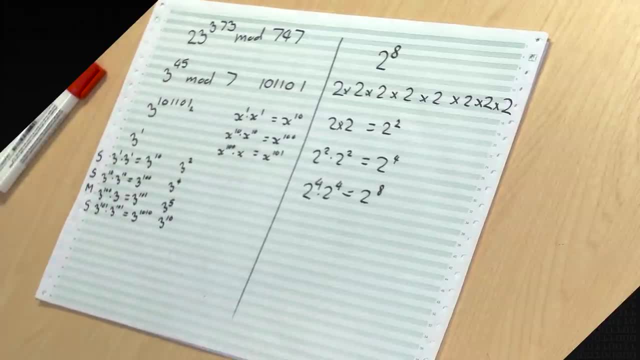 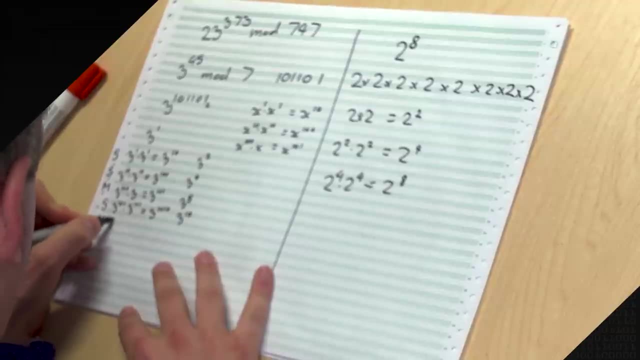 That's 3 to the 10.. Right, And if anyone's got their binary calculator out, you can confirm my working here. Right, Let's keep going. So we're going to multiply, So 3 to the 1, 0, 1, 0.. 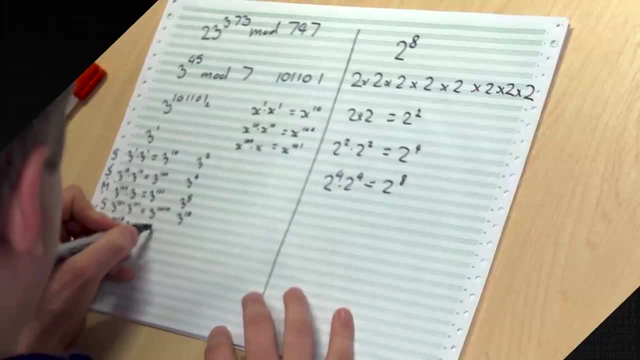 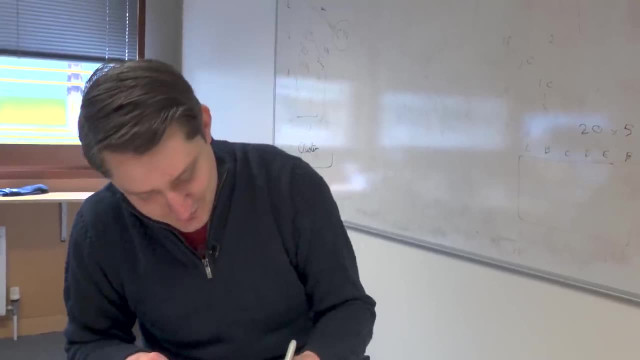 Multiplied by 3 is equal to 3 to the 1, 0, 1, 1.. So we've now built up the first four bits of our exponent. We're not that far away, I think That's 3 to the 11.. 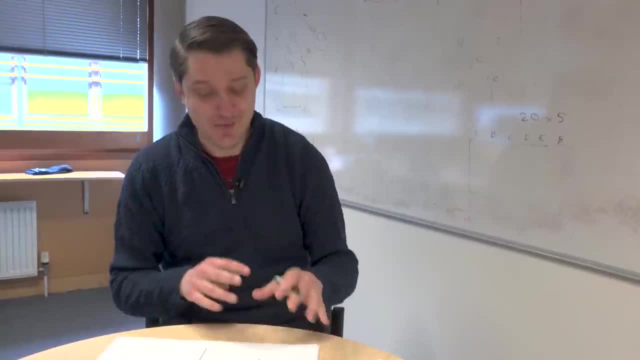 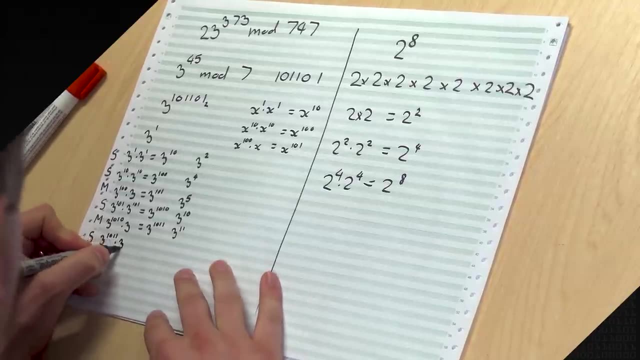 11 is nowhere near 45.. You're talking nonsense. We're nearly there. We've got to square it right. So 3 to the 1, 0, 1, 1 multiplied by. I should have just written squared, but then I would. 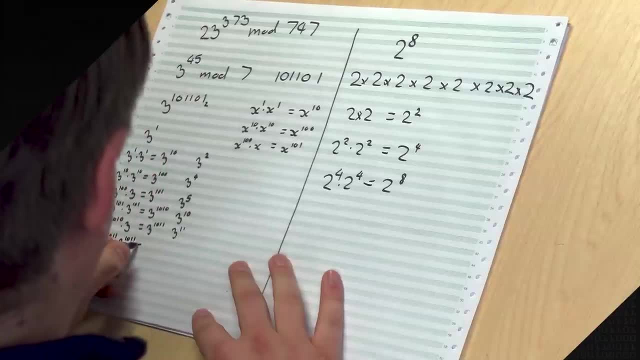 have had a lot of little numbers floating about, It would have got a bit confusing. 1 0 1 1 is 3 to the 1 0 1 1 0. Which is 3 to the 22.. 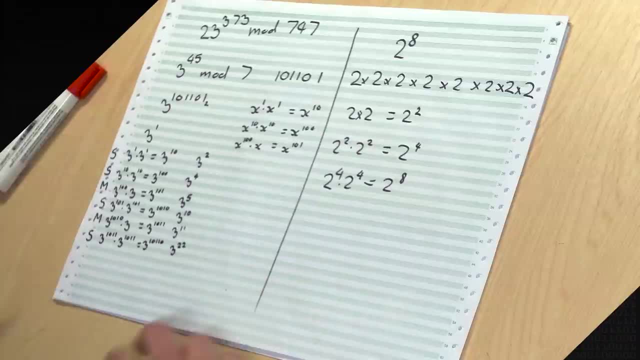 We've now got the first five bits of our exponent And now we need one last bit, So that's going to be a multiply. Oh sorry, no Square. Yeah, Yeah, Yeah, My bad, Square, Skip that step. 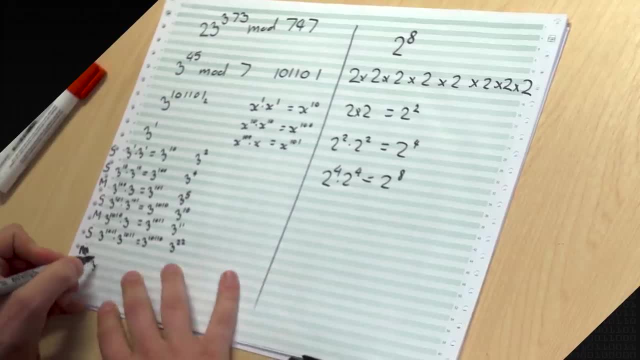 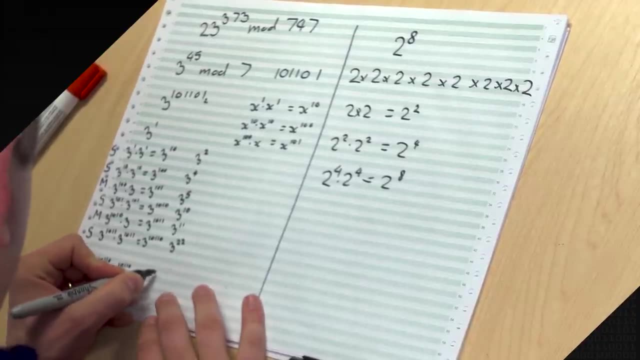 We pretend that step didn't happen. This is why you use libraries to do this, like Wolfram Alpha, and you don't use my implementation. So that's 3 to the 1 0, 1 1 0 times 3 to the 1 0, 1 1 0 is 3 to the 1 0, 1, 1 0 0, which is 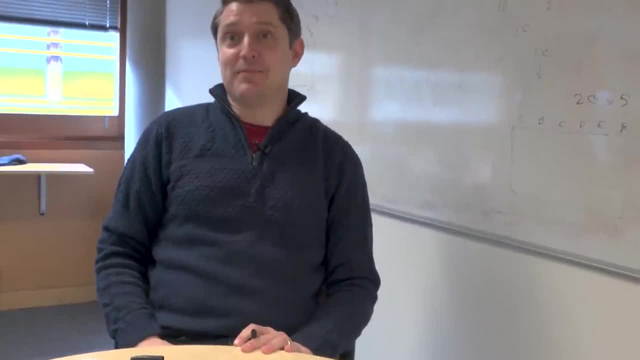 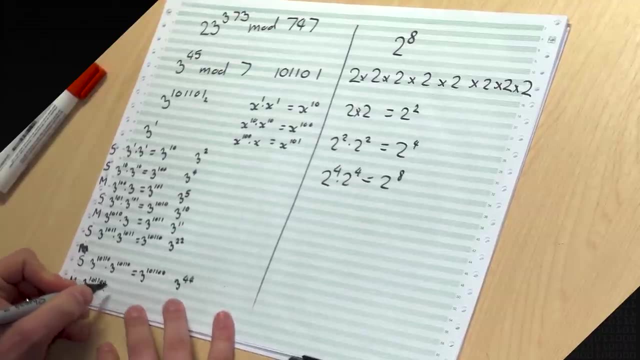 3 to the 44.. Now I think we're nearly there. right, Looks pretty good. We're just going to multiply one more time our intermediate value of 3 1 0, 1 1 0, 0 times by 3 to the 1,, which is the 1 there. 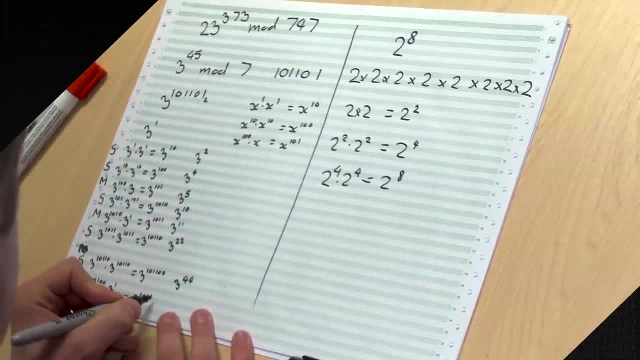 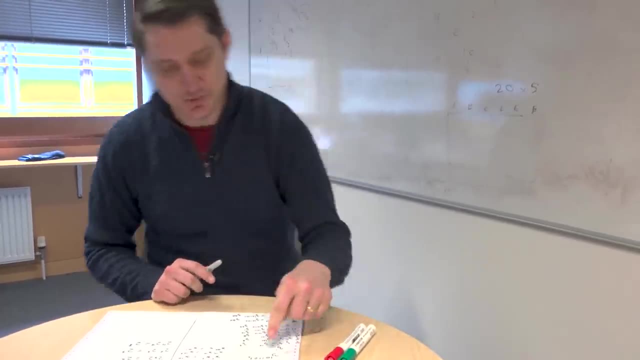 And that's going to be 3 to the 1 0, 1, 1 0 1, which is 3 to the 45.. Just enough paper. Just enough paper. Hopefully I don't need to add to this. I do actually. 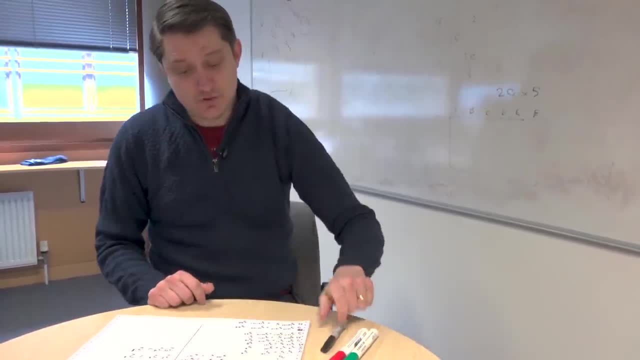 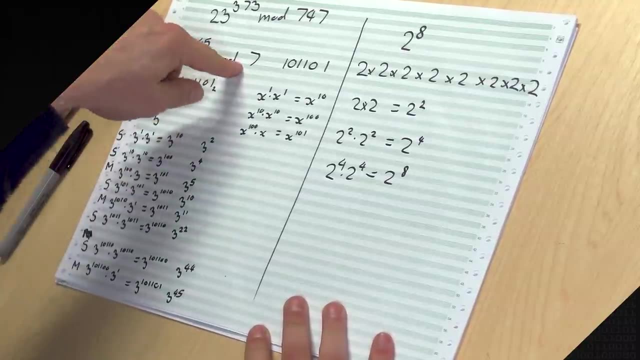 I wanted to calculate the actual sums right, But you know Now. So this is the exact combination we want. If we're doing this modular arithmetic, then every time we do one of these sums, we can reduce it modulo 7, and work out where it lands from 0 to 6.. 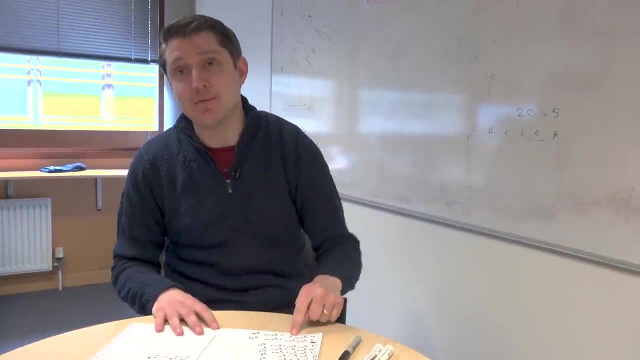 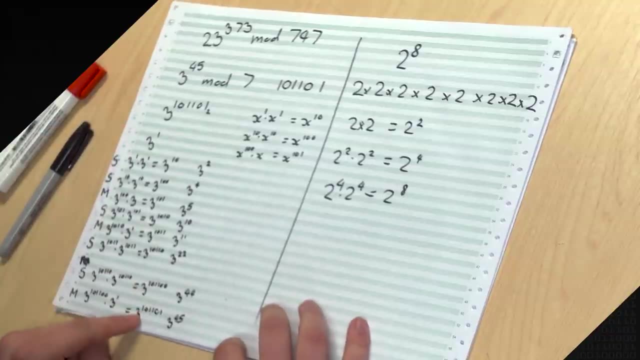 And that keeps our value very, very small. and we're also taking the exact minimum number of steps, So it's OK to remodulo it each time. Yes, So when you're taking modulo, all of these numbers end up as equivalent. 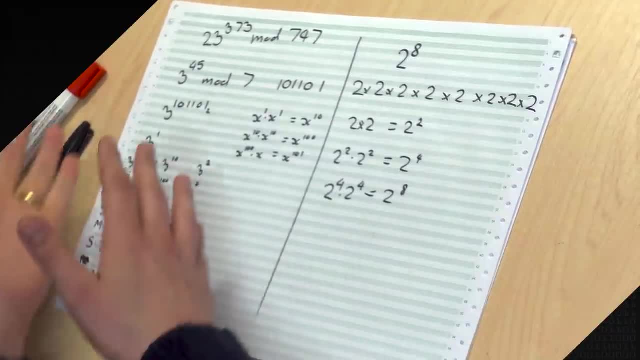 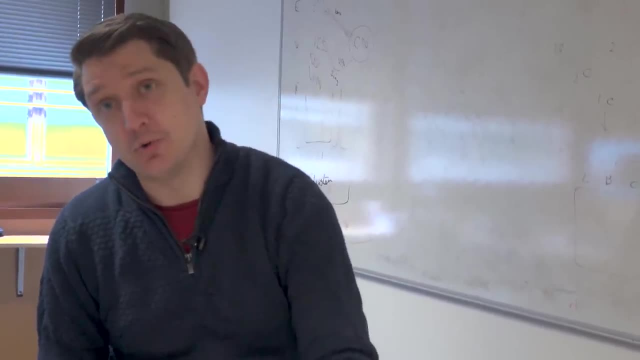 And so if you take mod all the time or you take it once at the end or halfway through and then once at the end, it doesn't make any difference. It will just change the size of the numbers. So in general, the rule would be that you do it as often as possible to keep your numbers. 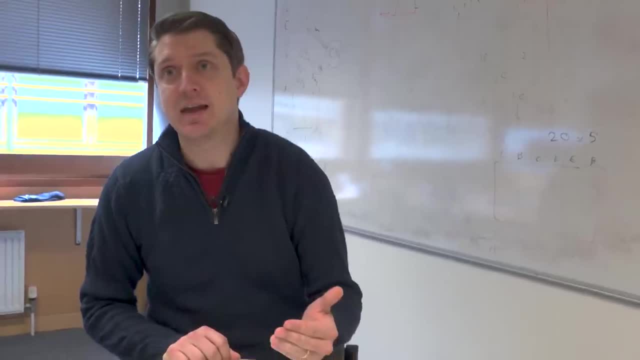 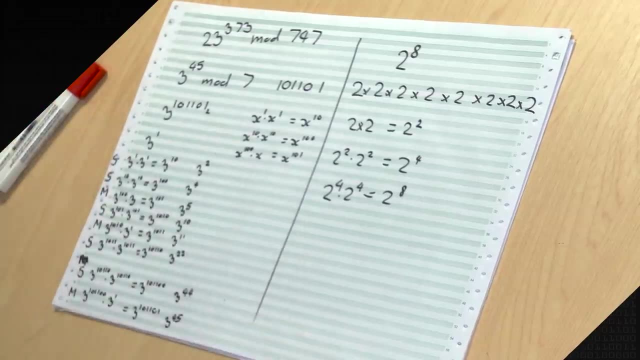 as small as possible. When you're multiplying numbers together, that scales very poorly with the size of a number, And so it's better to make them as small as possible. So let's actually work through this So we can just fill them in here. 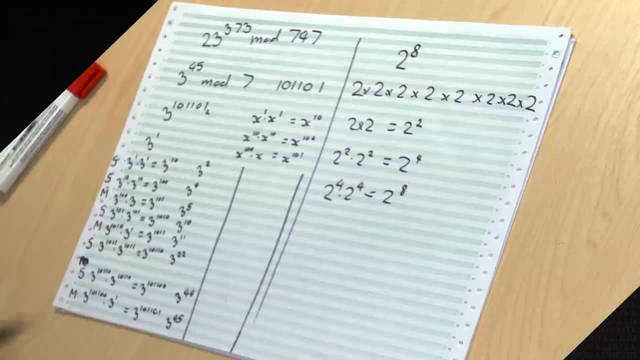 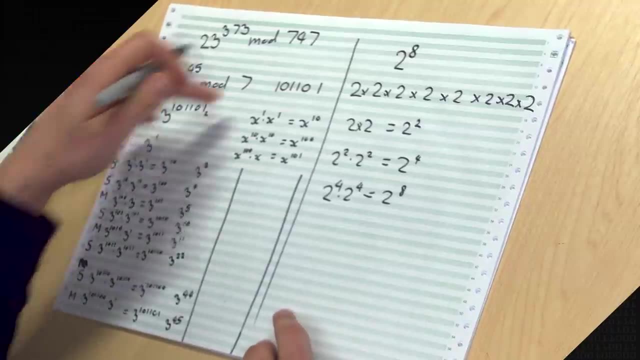 So if I just sort of create a little bit, This is the actual number we're going to calculate here, right? So the first one is 3 to the 1.. So that's our starting number here. You could start at 1 and multiply by 3 for your first bit. 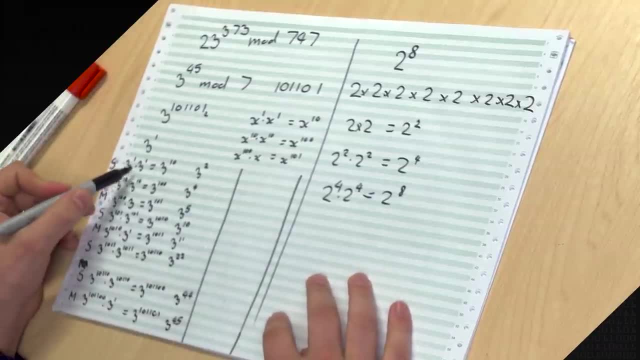 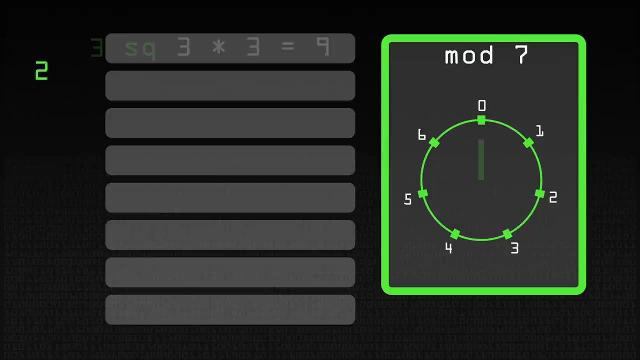 It's just an unnecessary step, Right? So the first thing we're going to do is 3 times 3, which is 9.. Mod 7 is 2.. Right, So that's 2.. Then this is going to be the intermediate value squared. 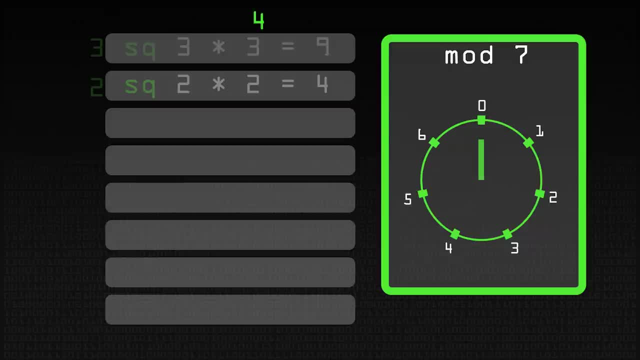 So 2 times 2 is 4.. Mod 7 is also 4.. Right 4 times another 3 is 12.. Mod 7 is 5.. Right, 5 times 5 is 25.. The next multiple of 7 below that is 21.. 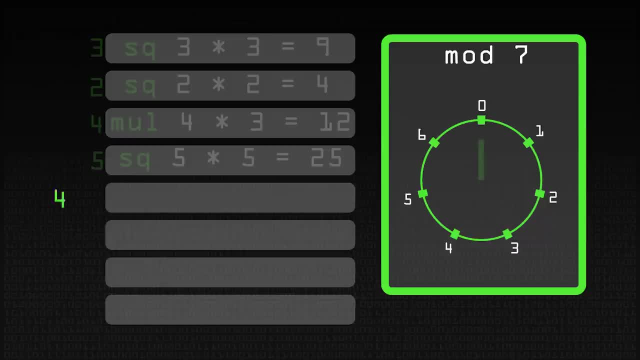 So it's 4, is the answer Right? 4 mod 7.. Right, It's not so interesting this one, So this is another 4 times 3.. We already did that, It's 5.. And then this is 5 squared. 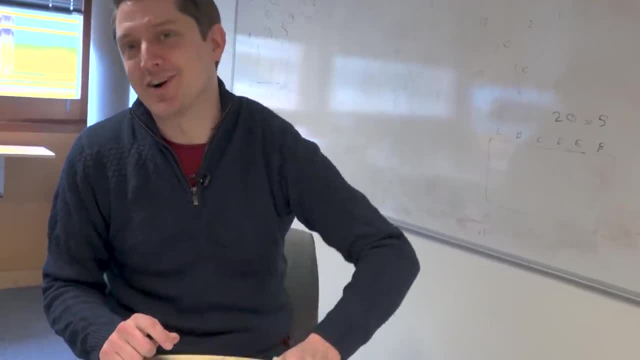 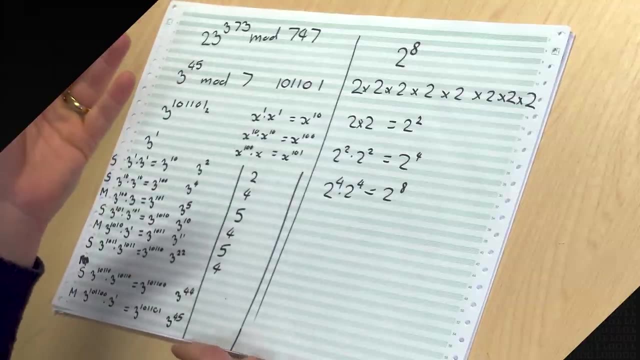 We already did that. It's 4.. You don't usually cache your results like I'm doing here. I'm cheating, Really finished. So now, 4 times 4 is 16.. Right, The next multiple of 7 below that is 14.. 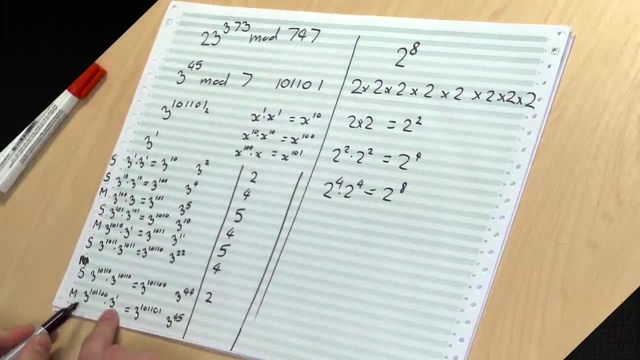 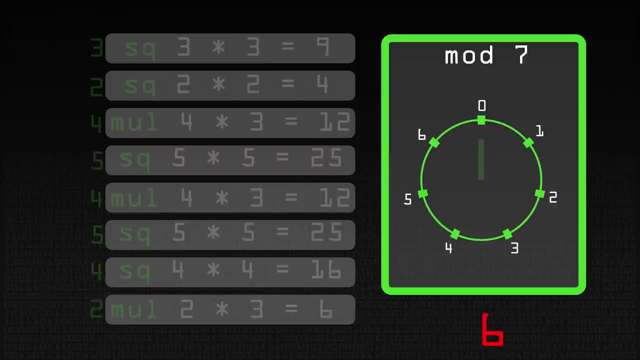 Right, So it's 2.. Right 2 times 3 is 6. And that's the answer. So if you do 3 to the power of 45, you get some sort of quadrillion or some really large number. 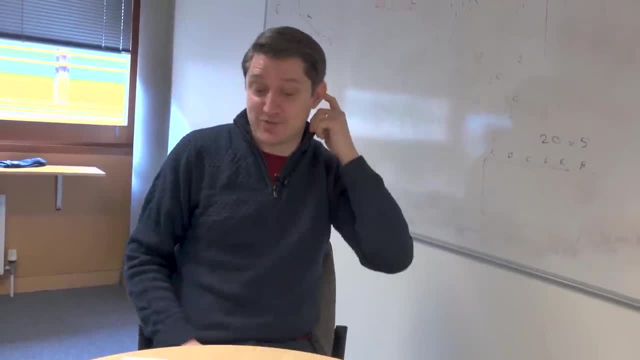 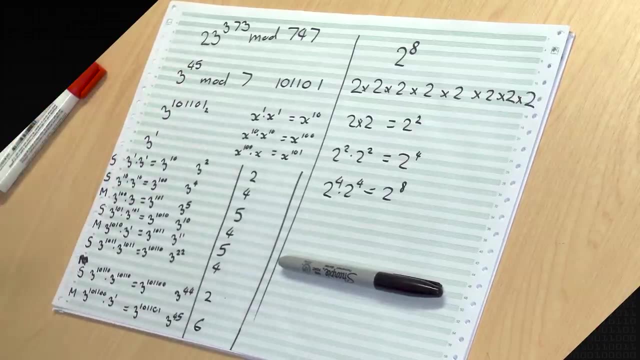 If you take it, mod 7,, 6.. Right, And we've saved quite a lot of memory and quite a lot of time doing this. We haven't had to do 45 multiplications, We haven't had to do very large intermediate values. 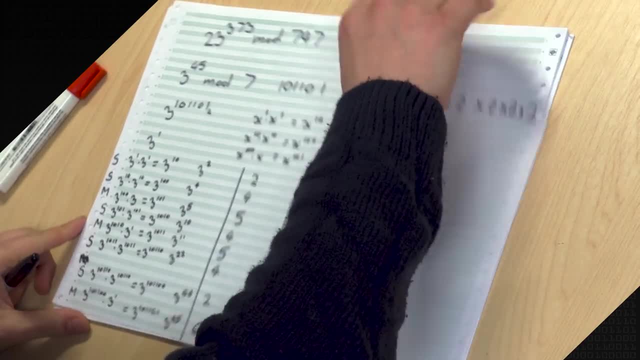 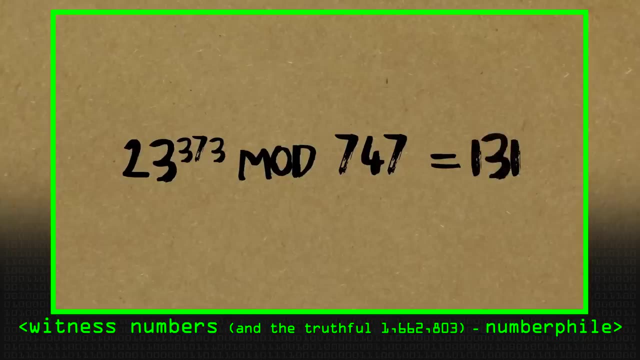 This is super useful for cryptography. Let's look at 23 to the power of 373 mod 747.. Now I think they calculated. the answer actually was 131.. I've run through this just to see if it works, And it does. 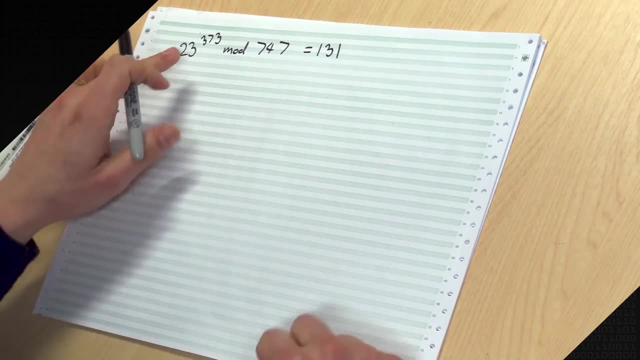 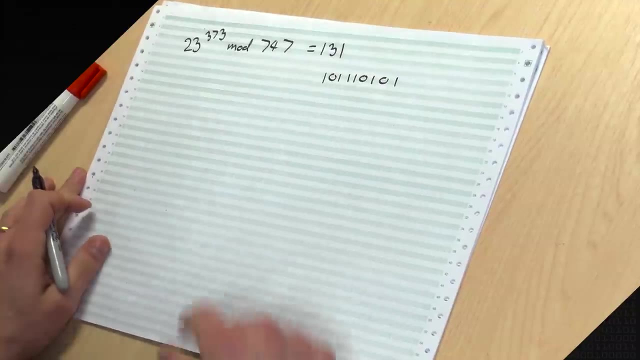 I can say that for sure, WolframAlpha's code is correct on this. But let's look at this: It's 373 in binary, Right? So that is 101 1 1 0, 1 0 1.. 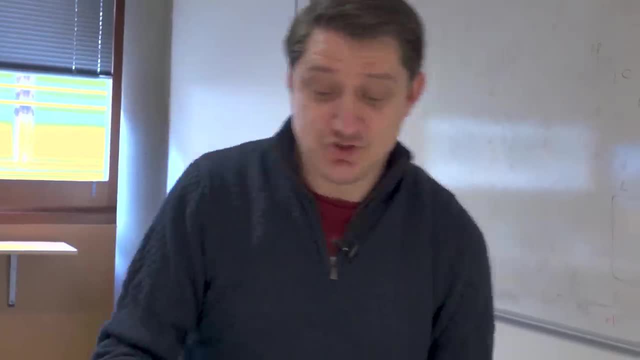 Which is quite long, Which is probably why I'm not going to run through it, So we could- actually I could- tell you what steps we need to do. So it's 23 to the 1. Right, That gives us our first one. 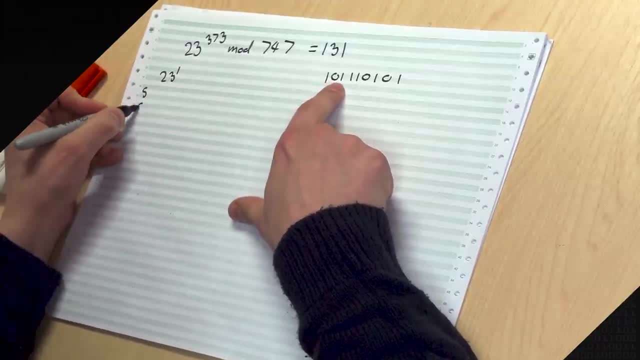 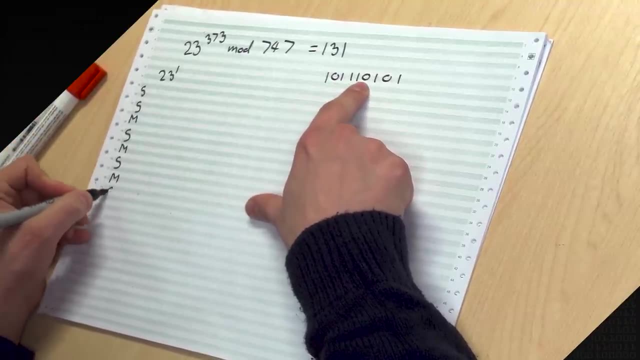 Then we're going to square, Then that will get us to here, Then we're going to square and multiply, And that will get us to the next one: Square and multiply. That's the next one: Square and multiply, Square, Square and multiply. 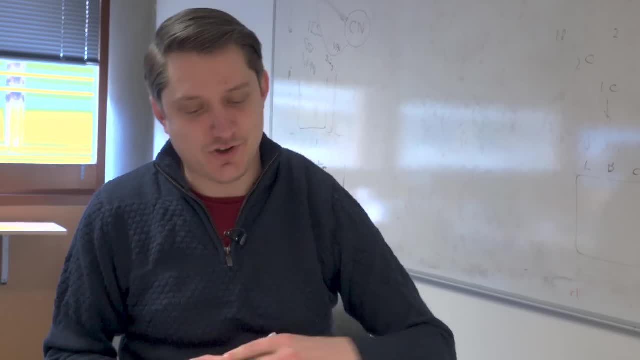 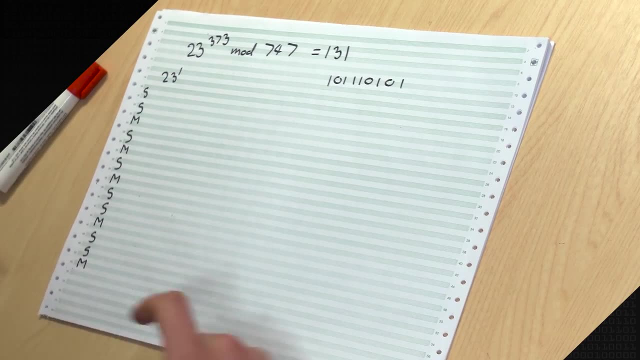 Square, Square, Square and multiply. Are you starting to work out why it's called the square and multiply algorithm? I think it's. yeah, It's something to do with squaring and maybe multiplication, So we could run through this. So if you square 23 to the 1, you get 23.. 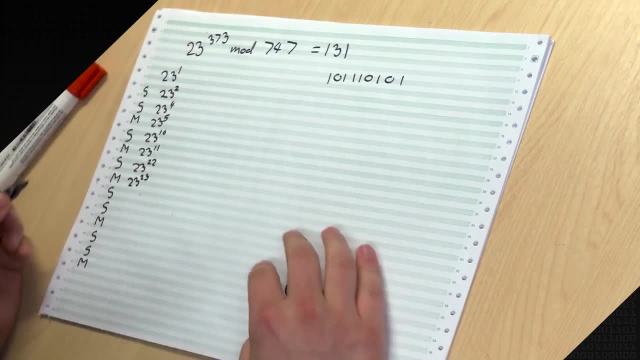 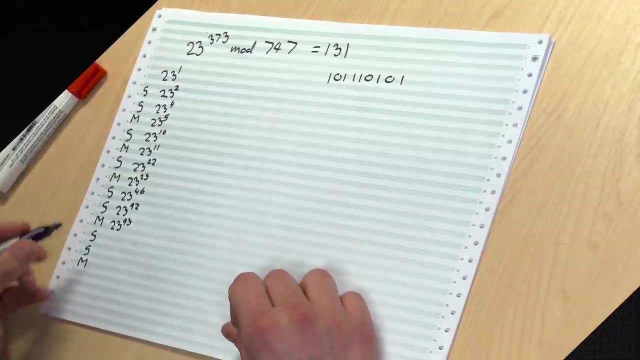 Keep going. So multiply 23 to the 23.. Square that 23 to the 23.. Now it's getting a bit hairy for me: 186.. 23 to the 186.. Square again 23 to the 286.. 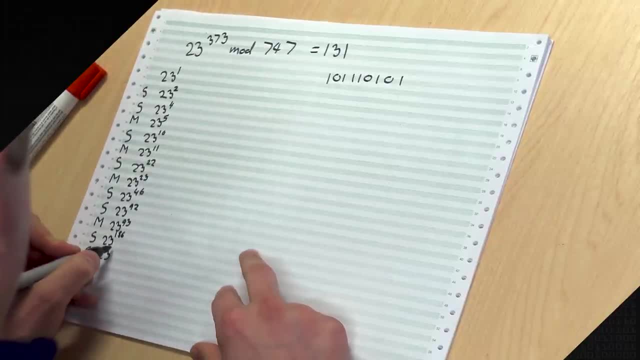 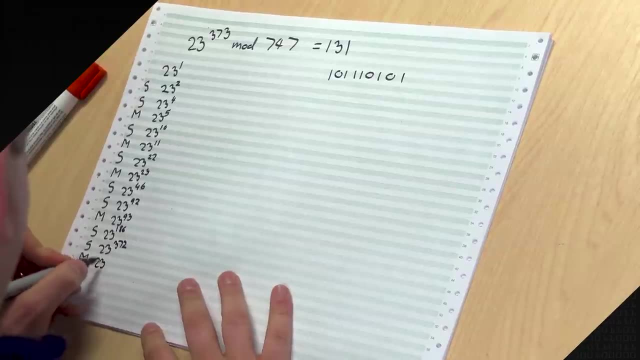 272.. 372.. That actually makes sense. That would make sense. I could have worked backwards, right, If only we could do that. 23 to the 373.. Right, So if you run through this on your calculator and calculate mod each time, you will hopefully. 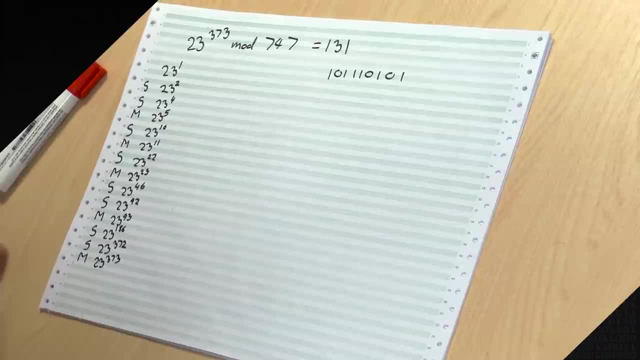 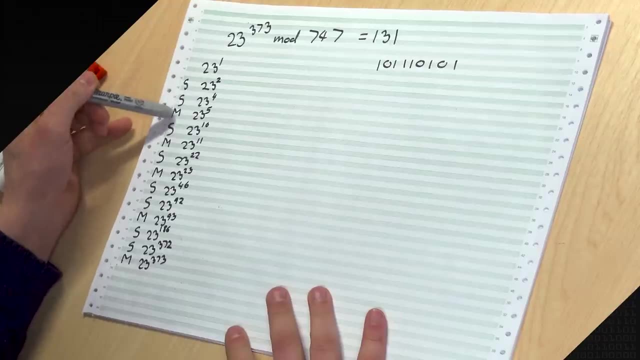 if you don't make a mistake, end up at 131.. This is actually quite a lot of steps. Let's see how many steps we've got here. So we've got 1, 2,, 3,, 4,, 5,, 6,, 7,, 8,, 9,, 10,, 11,, 12,, 13 steps. 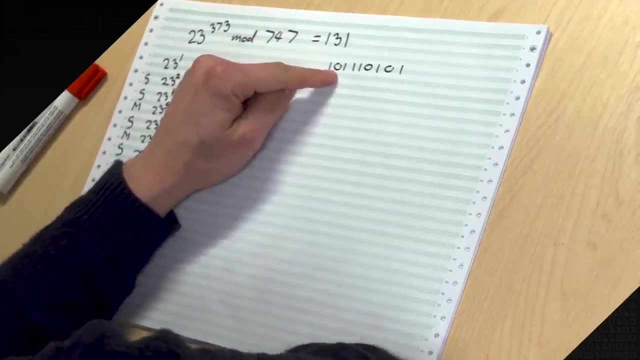 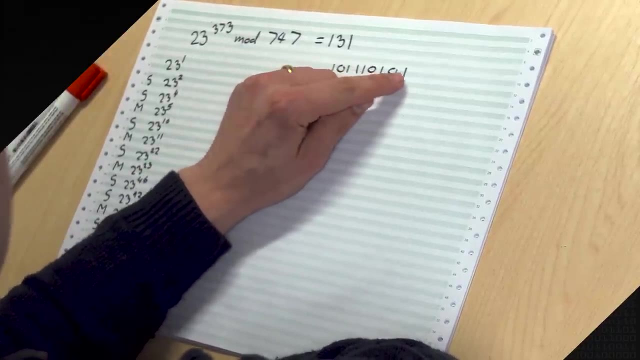 And actually that makes sense. For every 0 here we're going to need to do a square, And for every 1, we're going to need to do a square, followed by a multiply. So it's 1,, 2,, 3,, 4,, 5,, 6,, 7,, 8,, 9,, 10,, 11,, 12,, 13.. 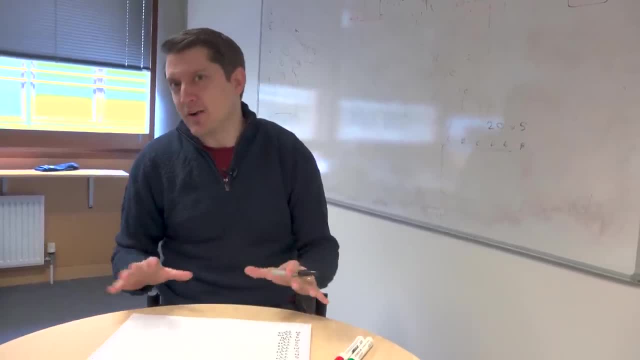 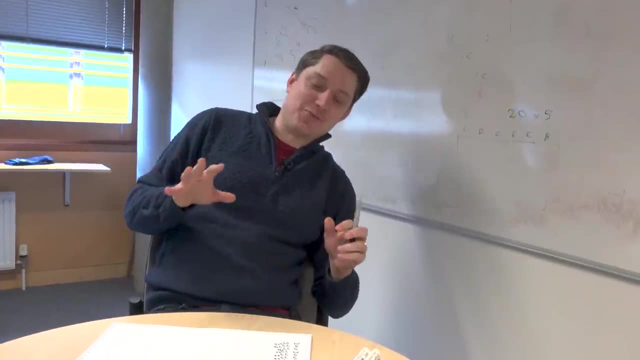 So you can see that, even for sort of 2,000-bit numbers, exactly how many squares and multipliers you're going to have to do is going to depend somewhat on the nature of this number. And that leads us to my last part, which is: I wanted to say that this is the best number that there is. 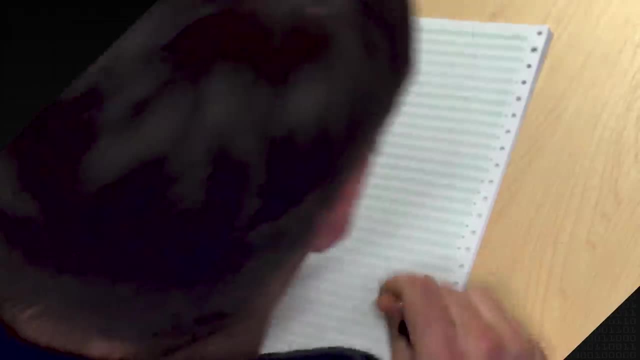 So this is 6, 5, 5,, 3, 7.. Now I for a long time thought this was the best number. Now I haven't been on Numberphile to explain why, But there is no doubt in my mind. 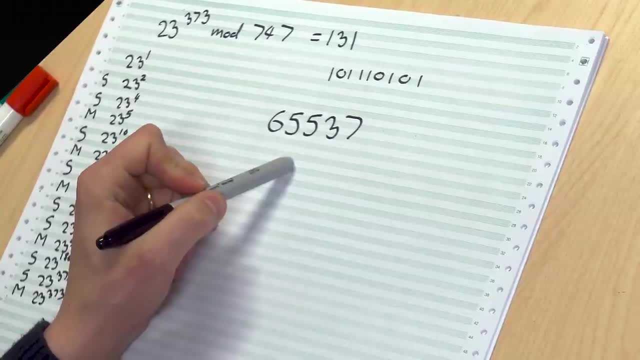 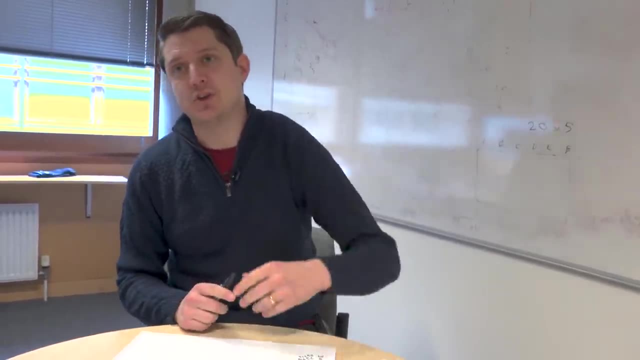 This number is used as the public key, which is the verification key, most of the time in the majority of RSA certificates. So on the web, when you go anywhere and a server gives you a certificate, the public key will be this number here and some large semi-prime number n. 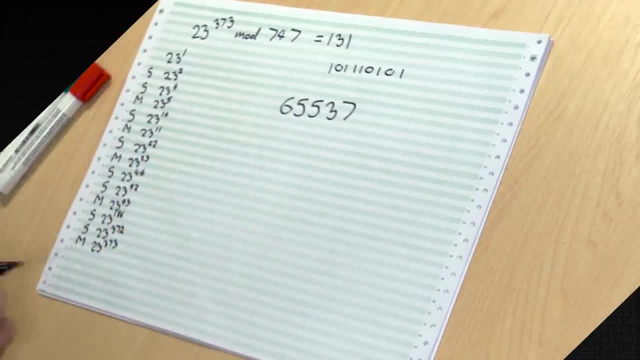 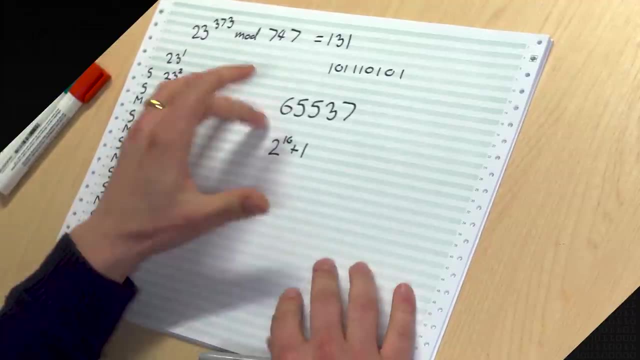 Now, why is this this? Well, if I write out the binary representation of this, this is 2 to the 16 plus 1.. Which also happens to be prime. Now, the reason it's useful that it's prime is because, mathematically then, 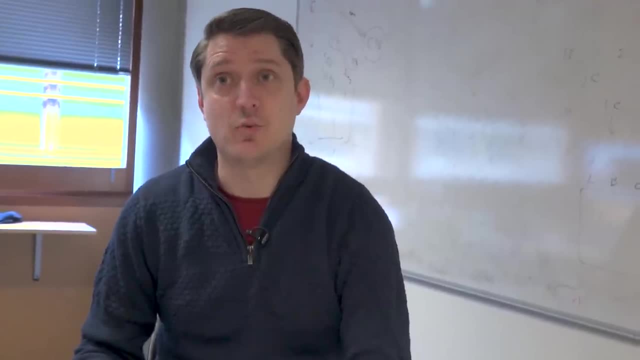 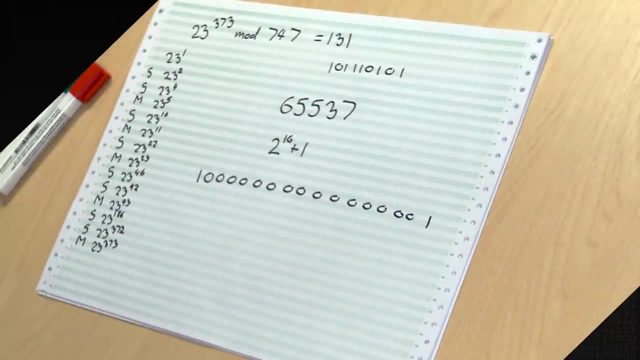 it doesn't share any divisors with another number, which perhaps we'll go into in a different video, But from my point of view, from this algorithm, the reason this is interesting is that it's the binary representation of that number In RSA. if you want to verify a signature, 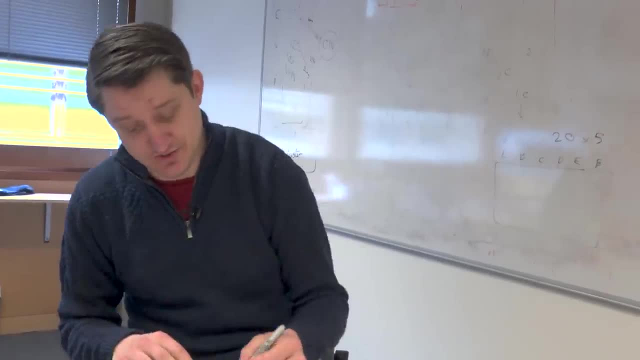 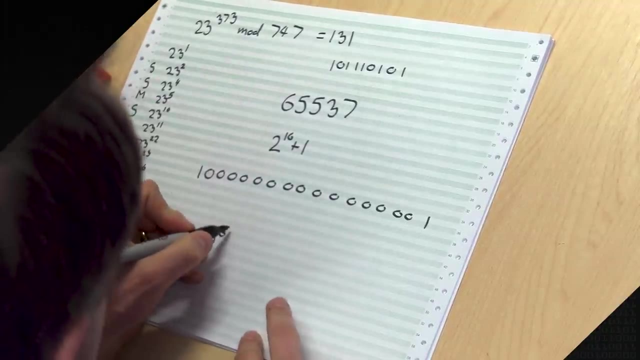 one of the things you'll do, beyond checking padding and a lot of other stuff, is you will calculate some message or some hash of a message, or some representation of a message, to the power of 605.. 655, 37.. 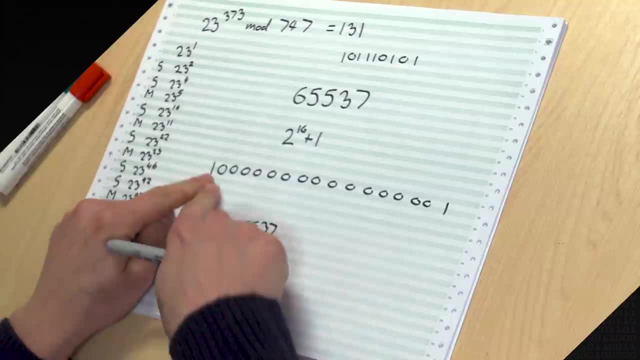 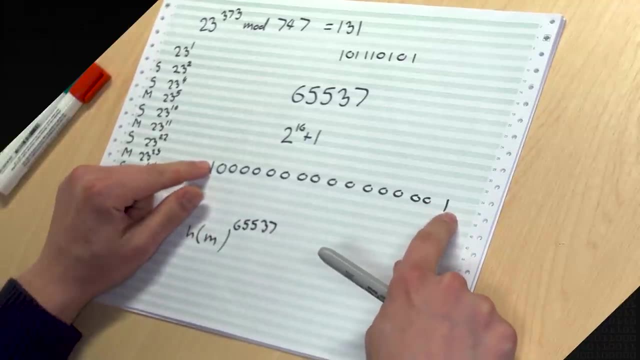 And that's going to be slow- Except it's not slow because there's hardly any ones in here. You start with one anyway. you do a bunch of squares and then you do one final multiplication at the end and you can verify very, very quickly. 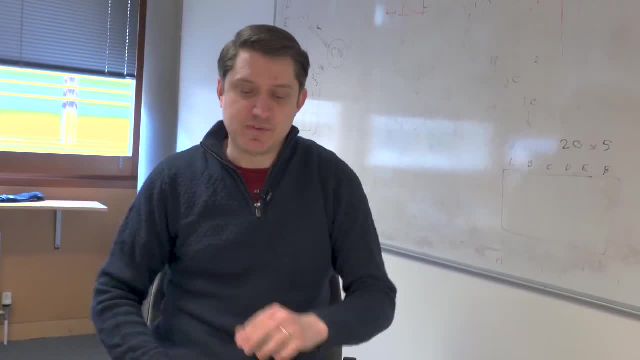 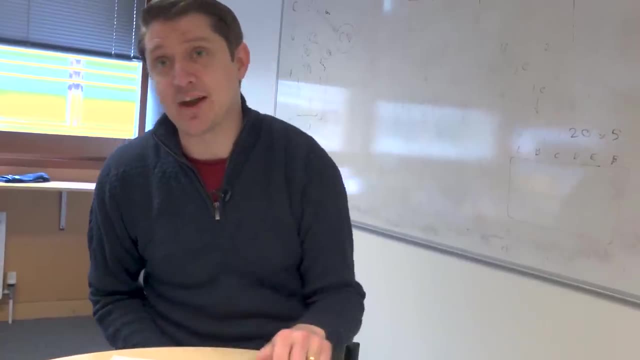 And that's actually one of the reasons that RSA is so popular. Even though elliptic curve signature schemes and other signature schemes exist, it's hard to beat the sheer speed of that verification process, which is what you have to do every time you go on a website or anything like this. 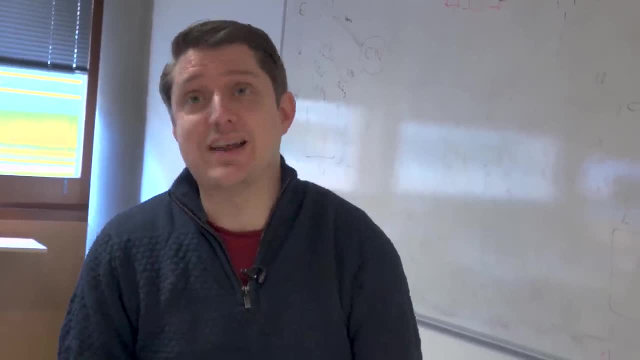 So it's a super useful function From a verification point of view. this is nice and efficient. Now, unfortunately, private keys tend to be much, much bigger than this, because otherwise they wouldn't be very secure, because you could guess them. 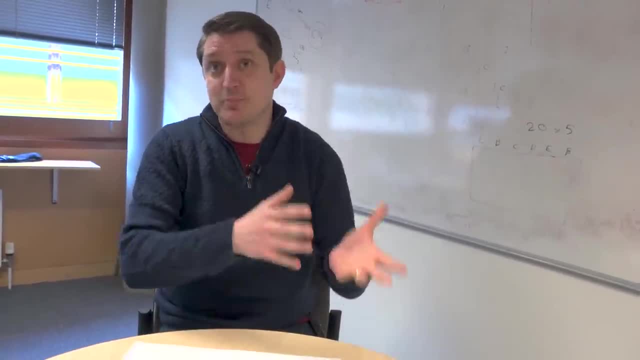 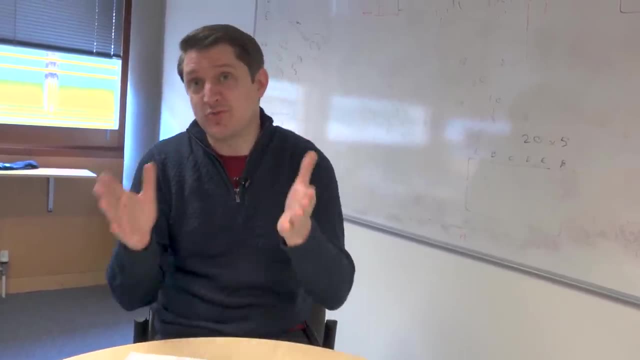 So you are going to be doing something like your message to the power of, or some message to the power of, a 2,000-bit number, But on average, you're going to do what sort of 2,000 bits? 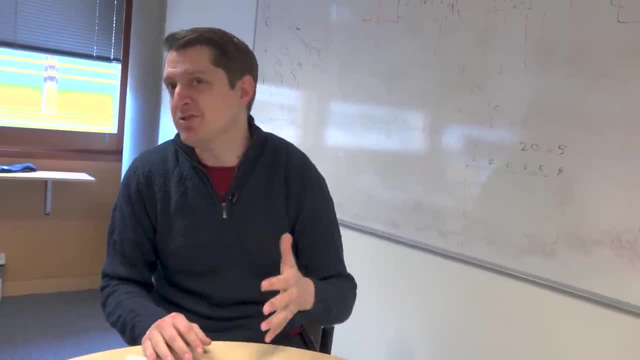 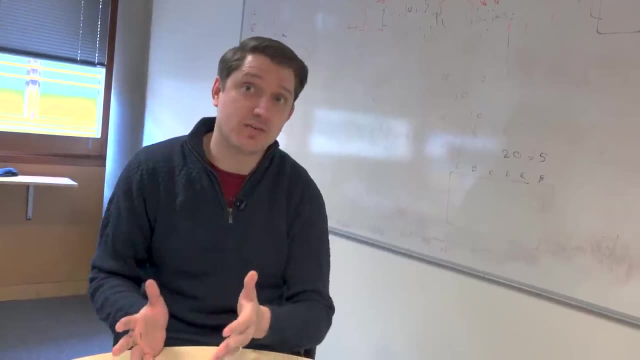 So that's 2,000 squares And then maybe half of them on average are ones, So it's maybe like one and a half the bit length, So maybe it's about 3,000.. So it's about 3,000 squares or multiplies. 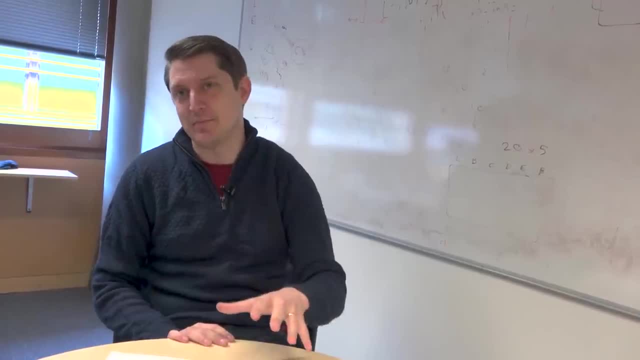 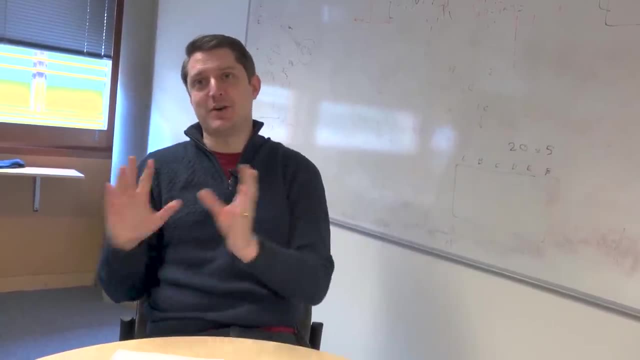 which on a modern computer is not so bad, It's not trivial. These are big, big sums But it's not ridiculous to imagine you could do it. Consider that if you did it the naive way where you did the message times by the message times, by the message 2 to the 2,000 times. 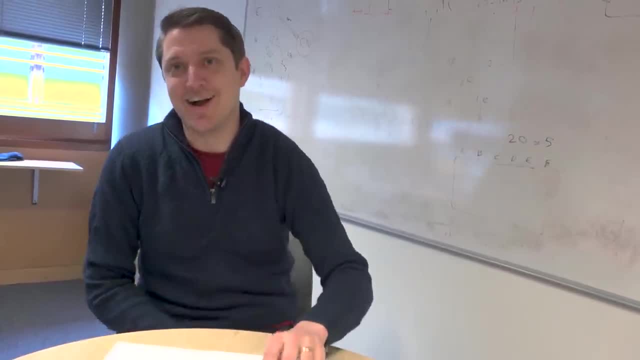 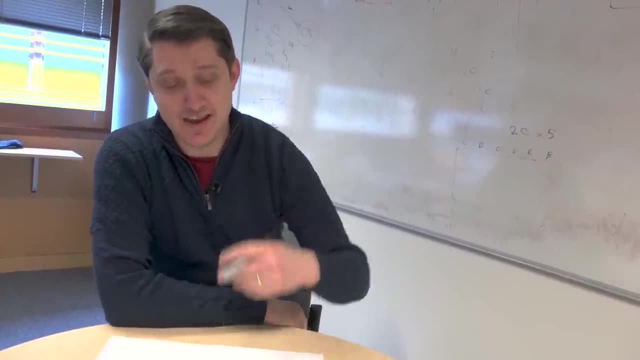 you would never finish in the lifetime of the universe kind of deal, So it's perhaps good that we have this. The only other thing I should mention, by the way, before someone corrects me in the comments if you use this for a private key. 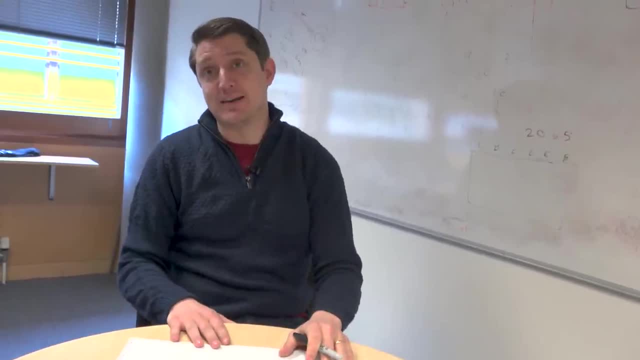 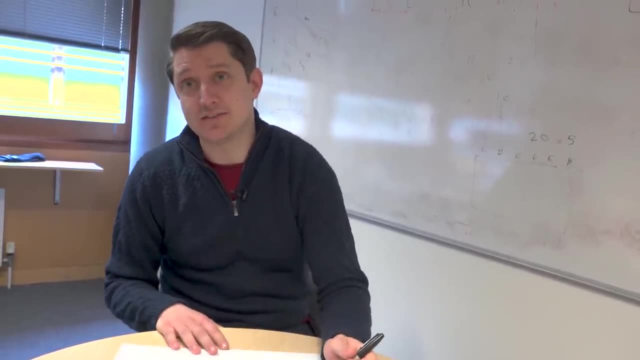 the problem you've got, then, is that the speed of your algorithm, and indeed even things like the power of your algorithm on the CPU, is dependent on what the private key is, Because you're going to be doing different amounts of square and multiply at different times. 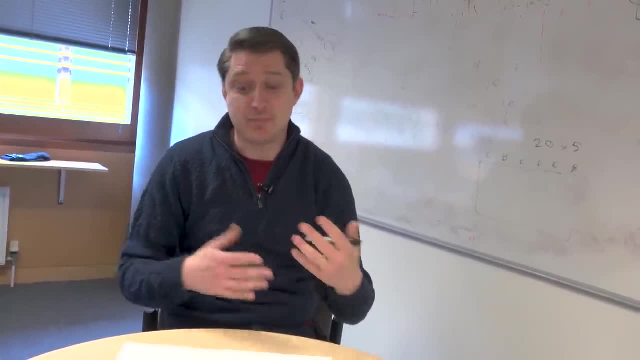 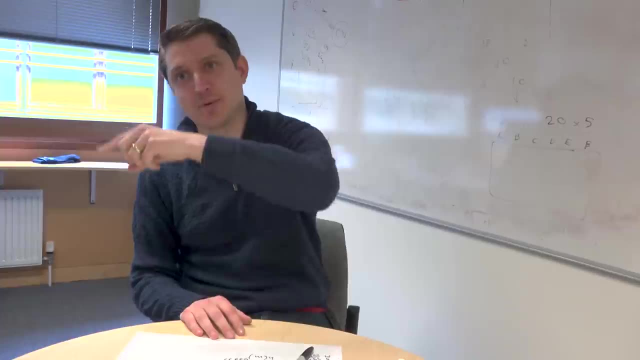 depending on the key. And so you leave yourself quite vulnerable to something like power analysis, where you can look at how much power drain there is on the CPU and you can see it go up for a square and then up for a multiply, and up for a square, and up for a multiply. 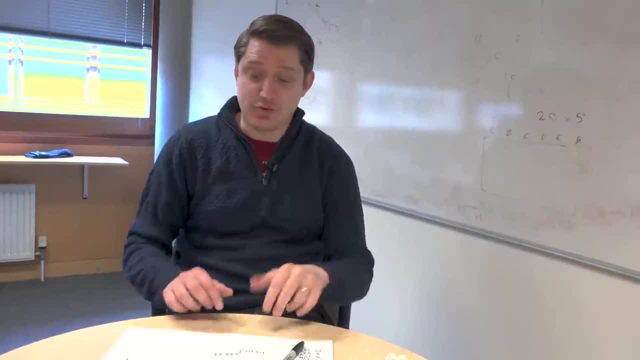 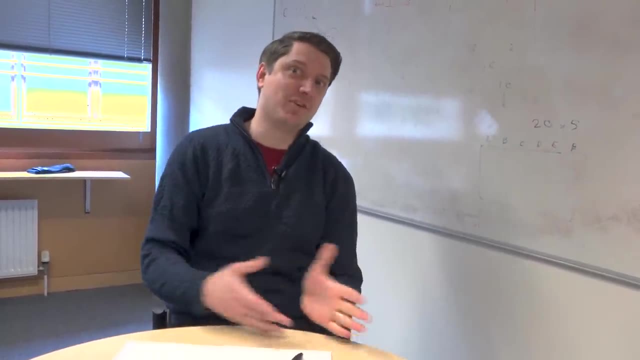 and actually just read off the key Right. And the other thing is that keys with lots of zeros will be quicker to use than keys with lots of ones in, And we don't really want to give away whether your key has a lot of zeros or a lot of ones.